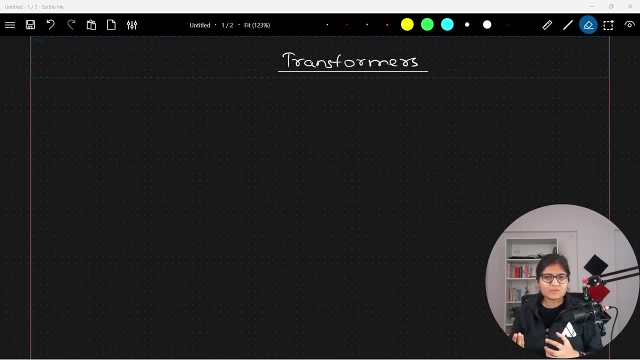 different architectures, But why? there is an advancement in transformers and nowadays, you know, apart from NLP, it is widely used in so many other applications. It is just because that the data set that is used in NLP is not used in NLP, So it is not used in NLP. So it is not used in NLP, So it. 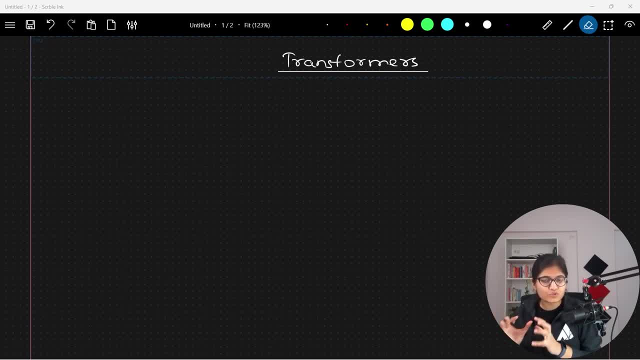 the data set that we have used, or the developers have used, to train the model is something which is quite vast, which is quite big, and that's why you know the results that we are getting from the transformers, which is a state of the art model in NLP. It is quite good as comparable to the other. 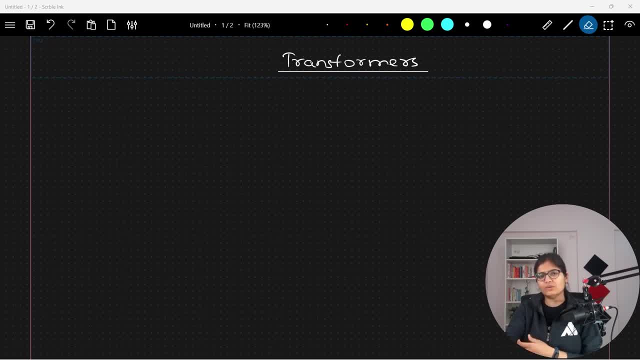 models that we have right. So I'll talk about a very basic application which we are using nowadays quite frequently, and i hope that you must have used this language translation. i hope you all know, right, what is language translation. so, in language translation, if you observe what will happen, for example, i am the person who just knows. 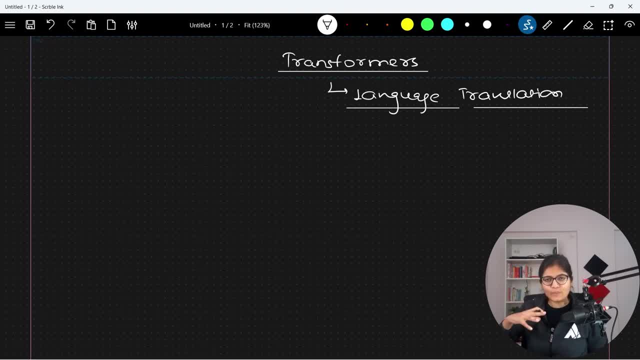 hindi language. i want to translate that language from hindi to english because i am in a country- maybe in us who, and with the people who are not aware about hindi language, so usually that is the only alternative that i have where i can convert via a mobile phone or google translator to hindi. 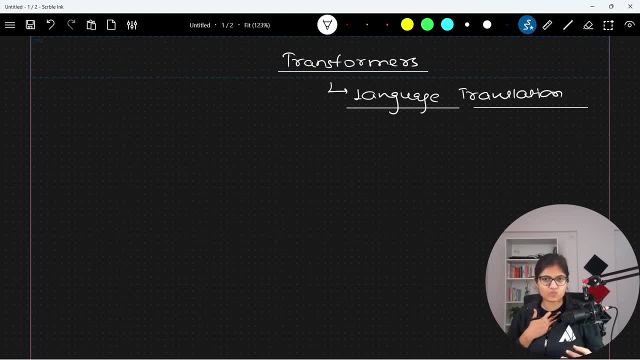 to english, for example, i am saying in hindi. so what will happen is that, whatever be the hindi word sent or the sentence that you are saying here, that you have, so what will happen is you will pass this hindi word to something which i would say is the transformer based model. 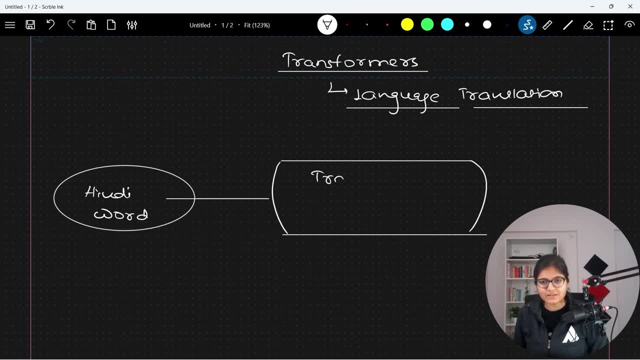 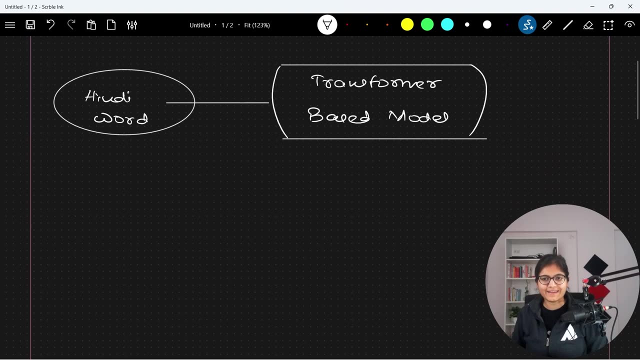 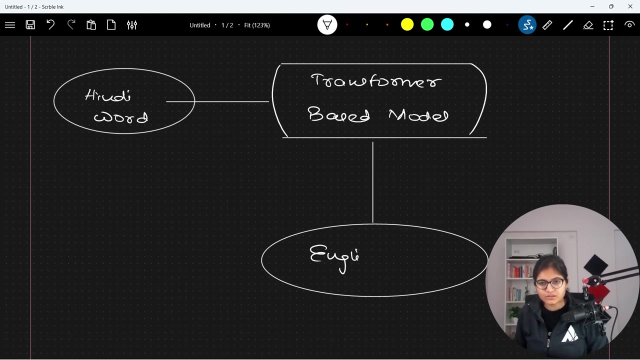 so something that i am saying is the transformer based model. now, what this transformer based model will do, it will try to convert whatever hindi word or the sentence that you said like to something that we are saying into a english word, into a english word. so when i am saying 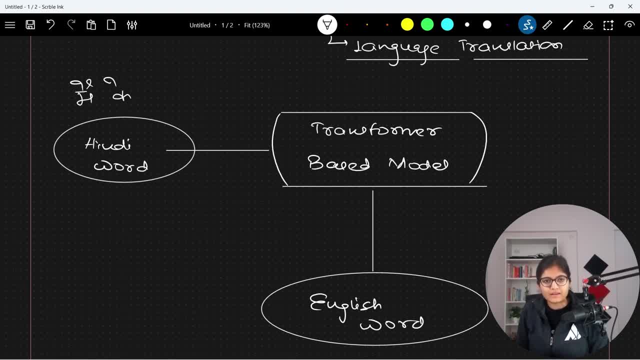 i don't know much hindi because i am writing quite after a long time, so suppose, so it is converting that transformer based model to a english word. that is, how are you? and that kind of development, that kind of translation happened just because of this transformer based model. so it is nothing, but it's a encode, decoder-based network, it's a. 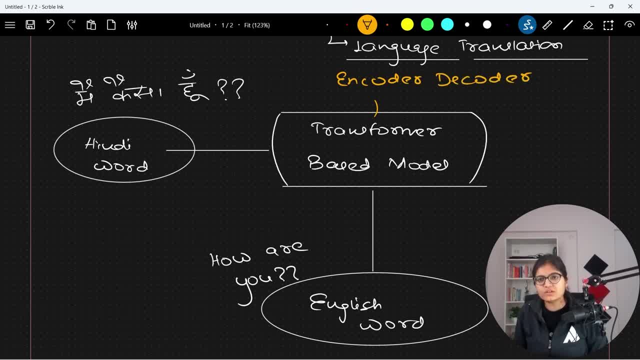 encoder, decoder-based network, where you will observe that in an encoder we are inserting the input. for example, in my case, in this present scenario, the input is my case. so what we are are inserting, we are inserting a input to the encoder. encoder will process that input. now 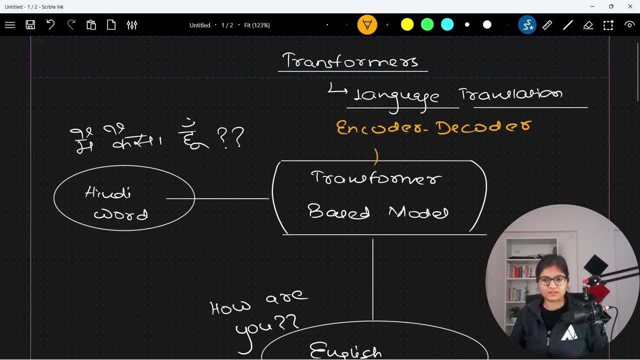 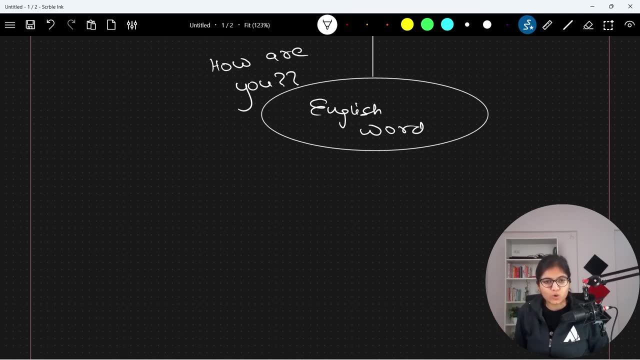 usually the very first paper which is uh developed by google people and tornado people is: attention is all you need, so it's developed in 2017, i believe there is a paper i i will suggest everyone, after this session, go and just have a look onto this paper by the name of attention. 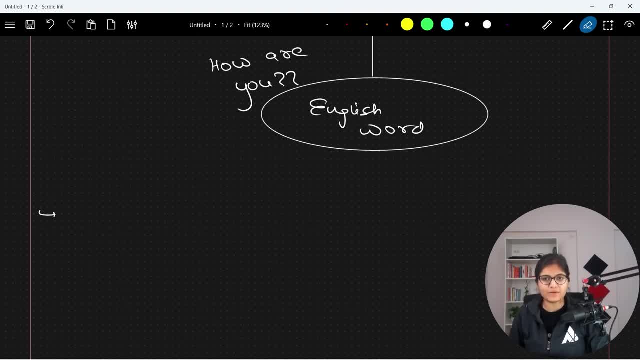 is all you need. i'm not sure why i am unable to write properly here. attention is all you need. just go and refer this paper. this paper was developed in 2017 and in this paper, for the first time, the transformer architecture was there. and that transformer architecture. 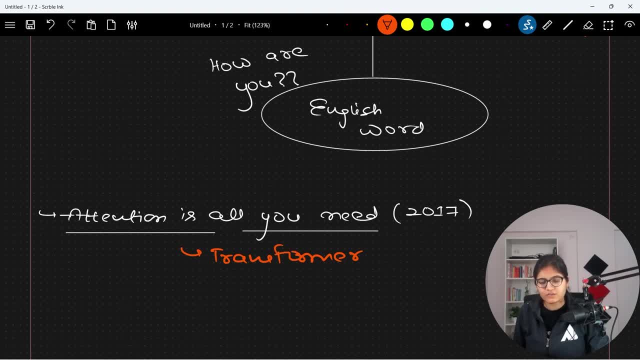 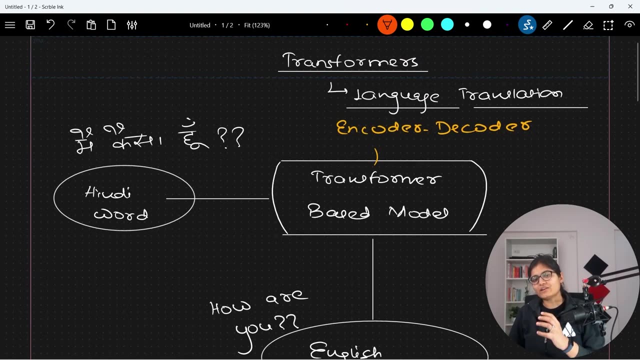 architecture, you will observe, is the one which we are talking about in today's session. So there is a complete transformer model architecture which you will be easily able to see in this particular paper. So what I am saying is that that transformer architecture is nothing, but it's a encoder. 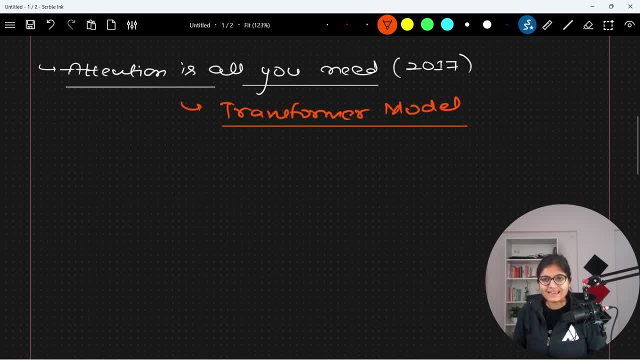 decoder based architecture where in an encoder. so it's a encoder, decoder based architecture where in an encoder we are passing a input. for example, in this particular problem, our input will be the Hindi sentence that we have passed. So here we are passing the input, then we will be having a layers of encoder and after that 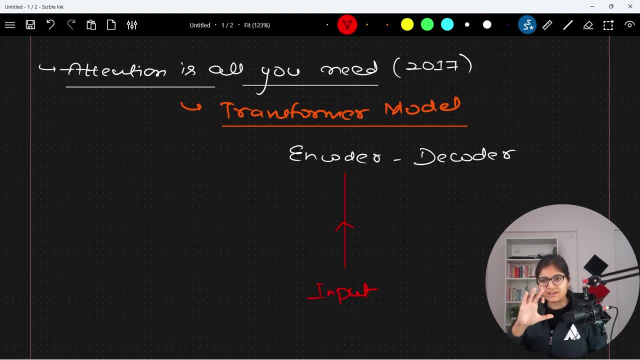 the final output Of encoder will be passed to the all the decoders and further the English sentence will be given by the decoder which is responsible to generate the output. This is how, basically, the encoder decoder architecture will be developed. initially it's a six layer based architecture, which you will see a stack of six layers of encoders and 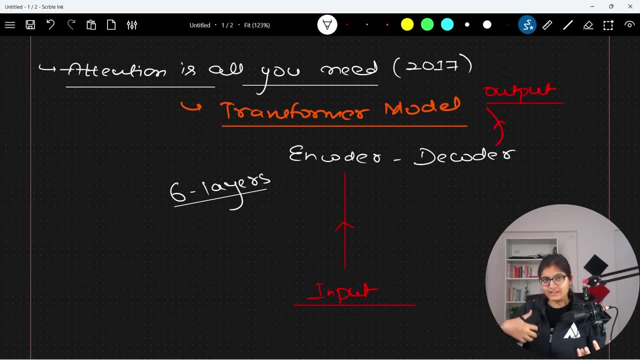 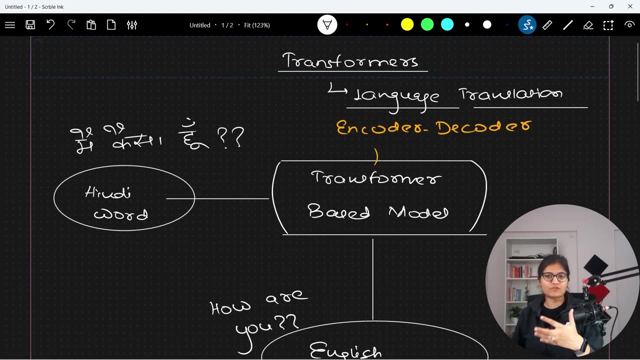 six layers of decoders. Encoder is taking the input, processing it and onto all the six layers of decoders- Six layers. final output of encoder will be passed to all the decoders that we have and finally the output will be generated. This is how the complete architecture of transformer will look like when you go and see the research. 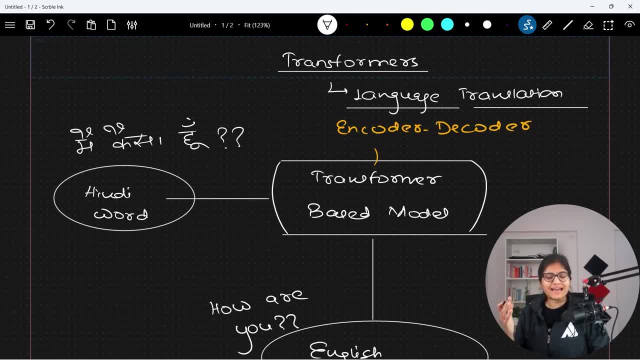 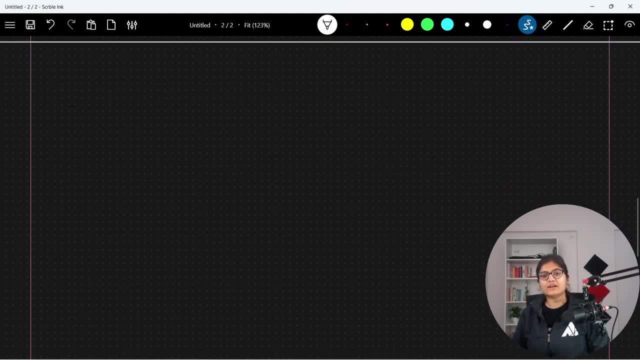 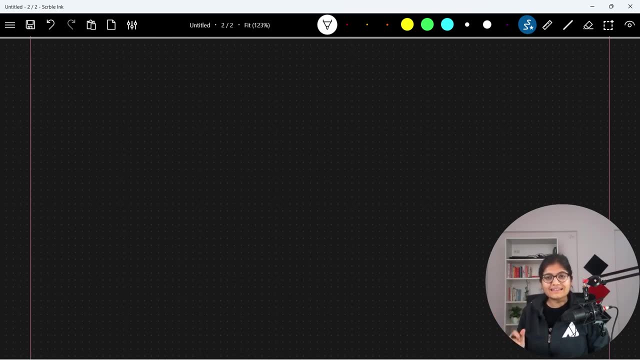 paper. But now, after some time, a lot of variants of this transformer came into picture. People or researchers started, you know, working very keenly towards the architectures of transformer. What they did is that they have taken completely only encoder portion, a stack of only encoders. 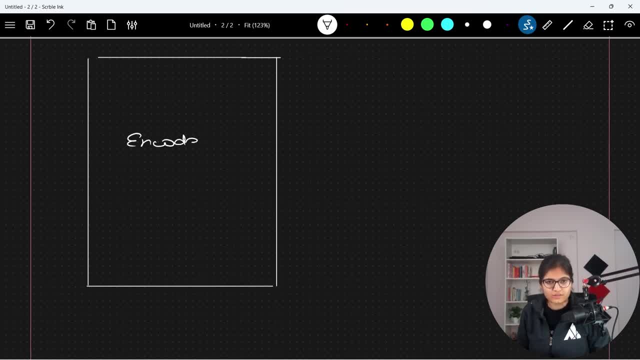 Now, layers will vary, so I am just writing a stack of encoders. a stack of encoders. Now, how many number of layers? it depends because there are so many architectures of transformers nowadays we have, and that's where the concept of BERT came into picture. 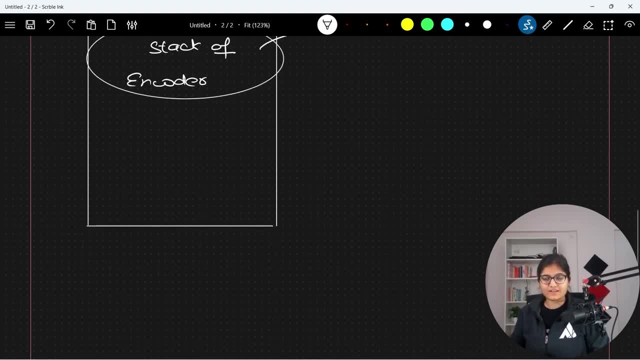 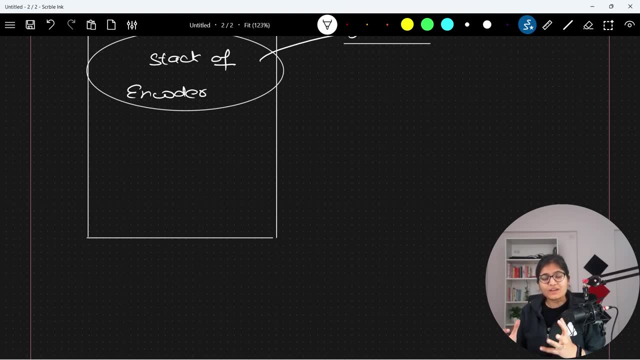 Similarly, there is another concept which, again, you have heard of, So everything is just a version of. you can say: transformer only where, if I take a stack of encoders itself, a different, different kinds of architectures has been developed by the name of BERT. Similarly, if I take only a stack of decoder, if I will take only a stack of decoder, anyone 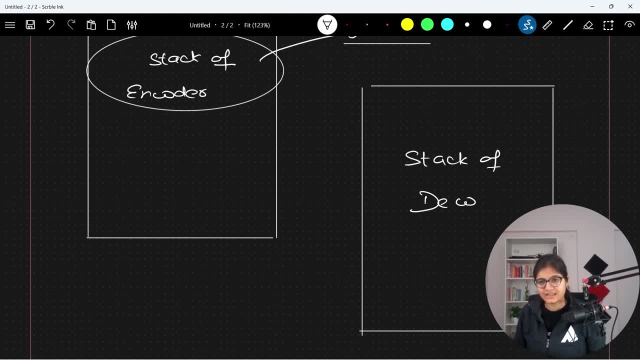 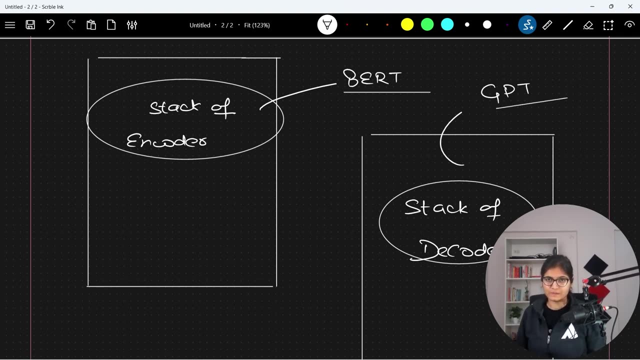 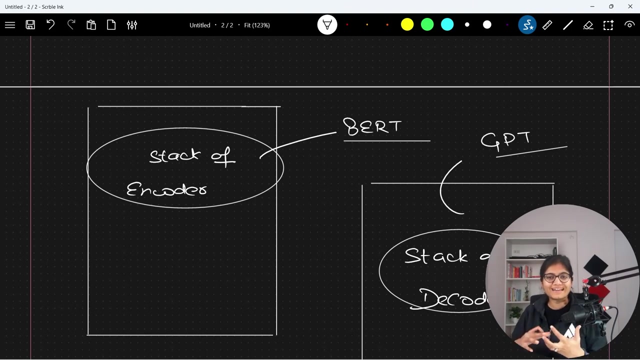 any idea What's that version of model is called as, where I am taking a stack of decoders present in the transformers and that is something that we called as GPT generative pre trained transformers. Now, why it is called generative? because here it is responsible to generate the context. 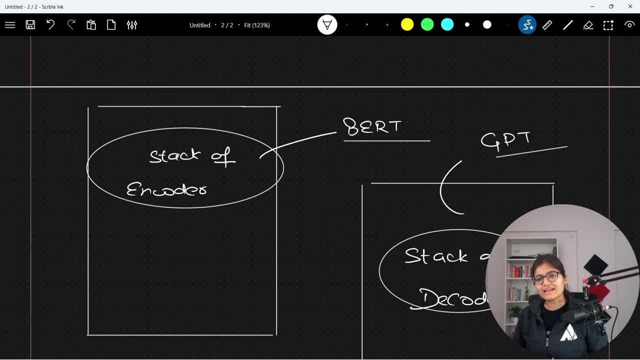 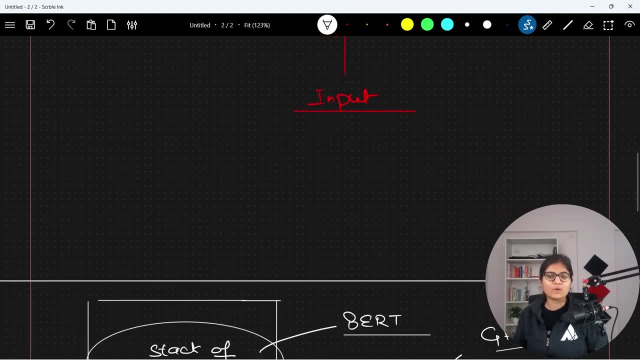 generate the text out of the given sentence, For example, That there are a lot of you know examples here. for example, if I will say once upon a time, what I want from my model is, my model will automatically complete that story. right, my model will complete that story. 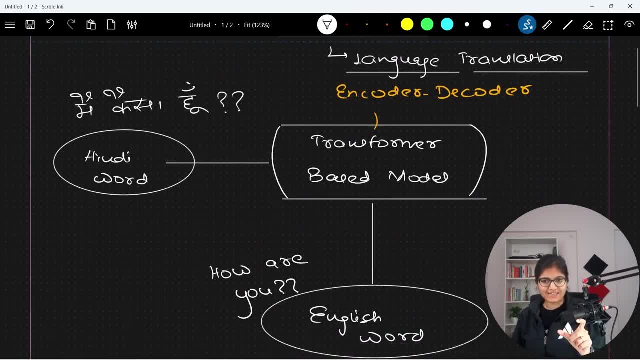 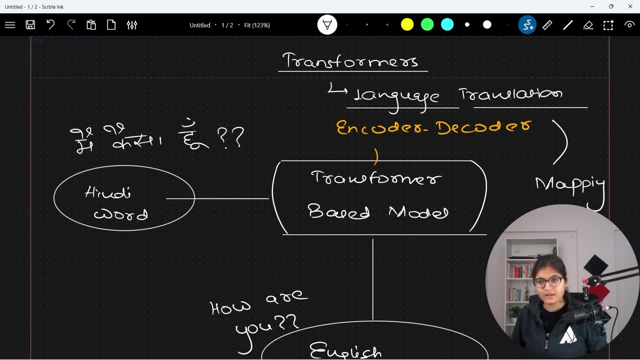 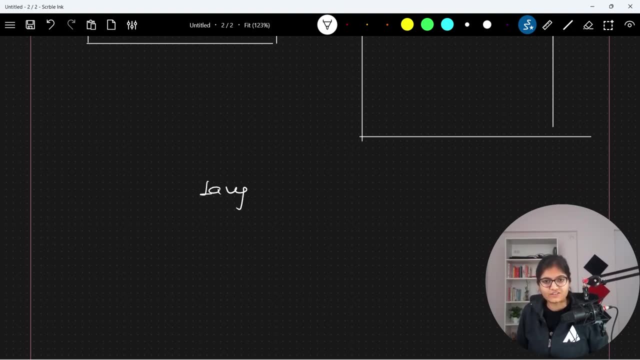 So in language translation which I just now talked about, one application here, somehow I would say, a mapping is required. Mapping of words is required, right. but the second example which I was talking about is the language generation task, And GPT is a language generation model. 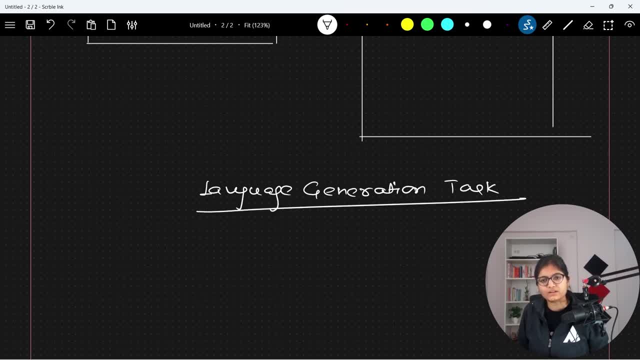 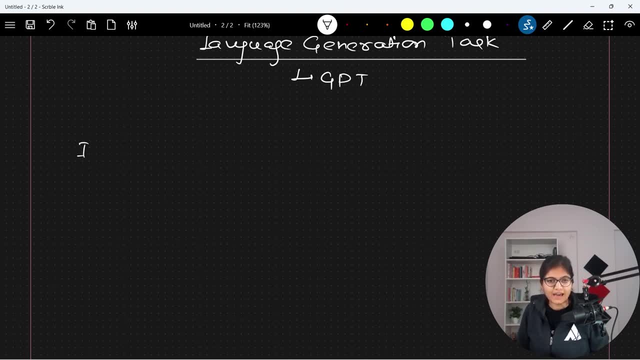 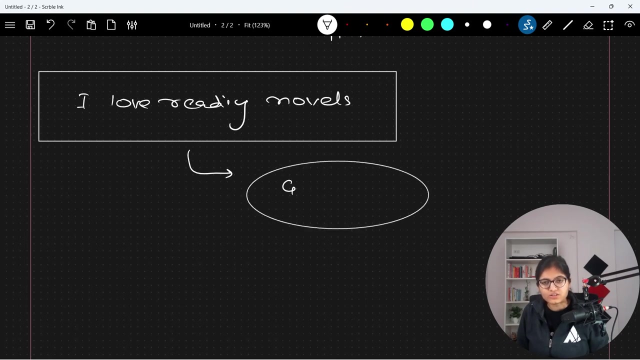 So in language generation task, where GPT plays a very important role here, what we want is, for example, if I will say that I love reading novels. So what I want is: given this is this as the input text. if I will pass this input text to: 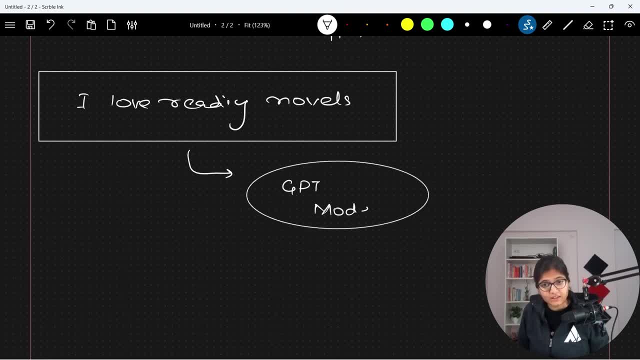 GPT model. now again, there are a lot of versions of GPT. you will see GPT 2,. you will see GPT 2 large. you will see GPT 2 medium, depending upon what kind of architecture that you are using. 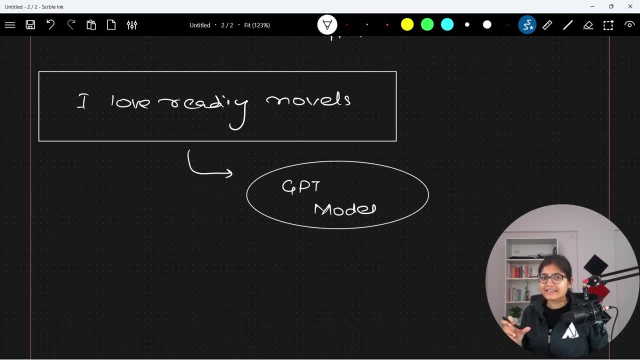 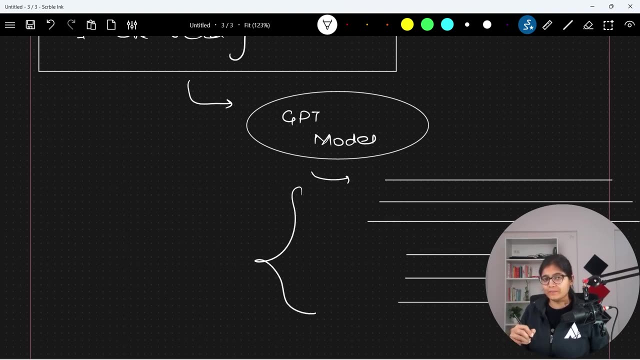 But fundamentals are same. But you will observe that for every architecture You are using a decoder, stack only what it will generate. It will generate a complete you know Story out of it, because you will observe that these GPT models have been trained on a huge amount of data set. 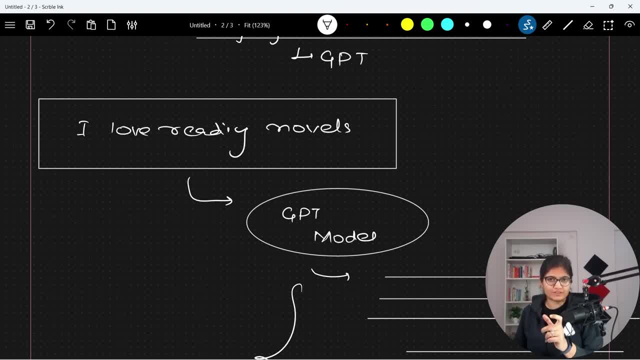 and that's why we are calling it as a pre-trained models, because the training is already been done on a huge amount of data set, with the help of which it is just trying to fetch the records, the data where this particular line resembles. So now here, you will be easily able to understand. 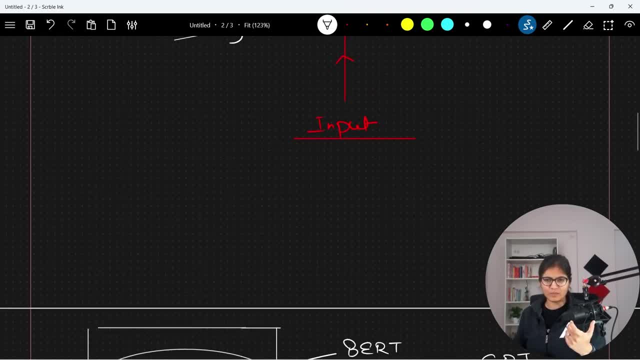 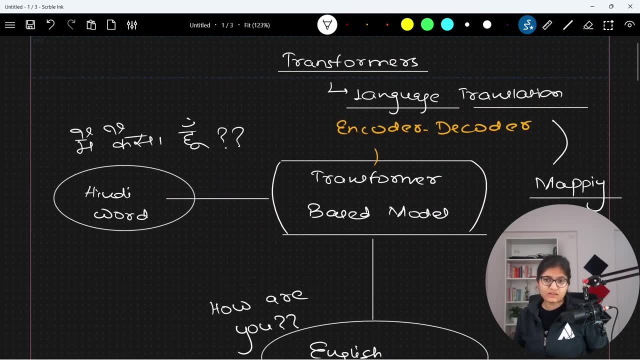 that somehow we will be having a transformer, which is we will be able to understand as an encoder, decoder type of architecture, where it is responsible for many of the real-time application tasks. One more example which I can give you is the auto completion task where, for example, you 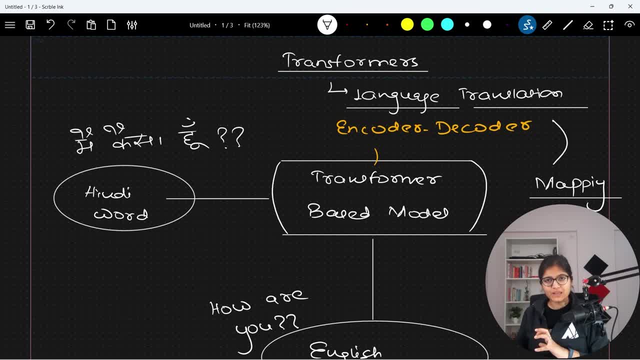 will observe that in the mails while writing, if you're writing something automatically further the points or the sentences, it is trying to give you auto suggestion there. All these are the application tasks. So now you will be able to understand that somehow we will be having a. 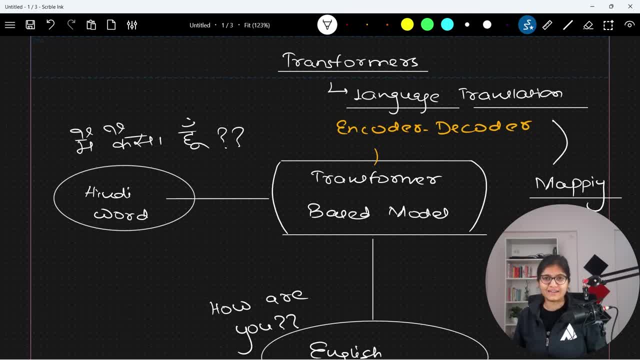 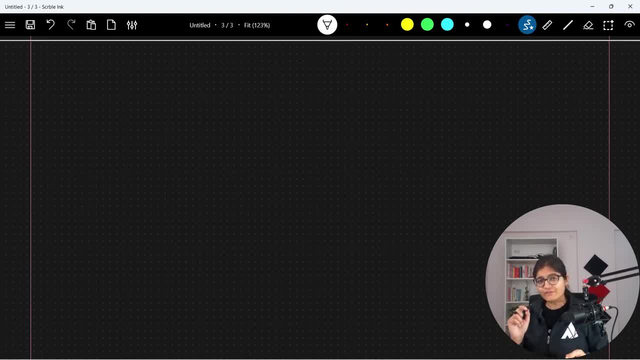 can ask from me, is that how it is going to work? The very first important thing is that you will observe, in the transformer architecture there is a component called attention. Again, that's a very important, you know, concept, but just I want to give you overview that what are the components that we 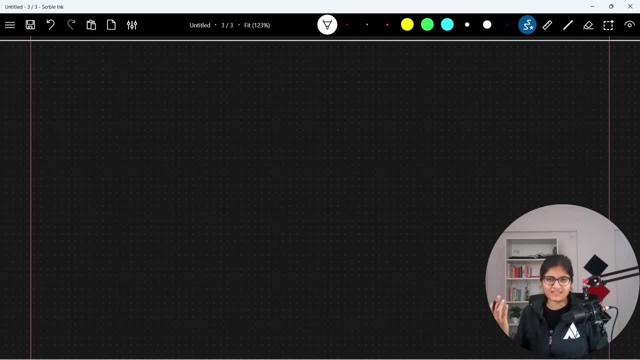 have in transformers. One is feed forward, which is nothing but is a multi-layer system. So you will observe that we have a deep learning. apart from that, you will observe that we will be having something called as attention. Something called as attention. What does that indicate? What is the? 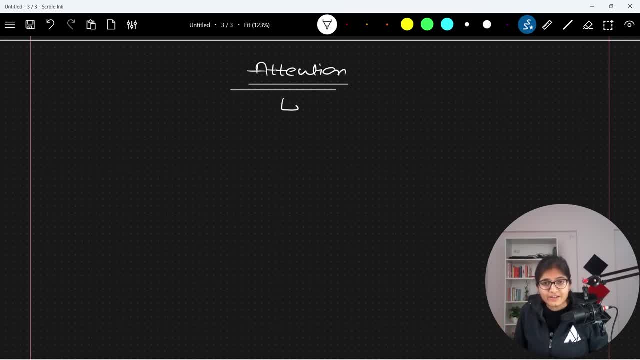 meaning of attention and why it is required. It is required to understand the context because if my model will not be able to understand the context, how it will be able to- you know- complete the sentence, whatever applications I am talking about right, or how it will be able to complete the sentence. 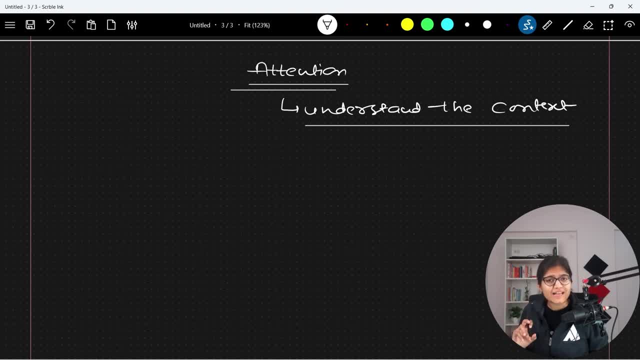 How it will be able to map and convert it into a proper English language, from Hindi to English, maybe from French to Hindi, anything. So understanding of context is the bigger problem In the initial cases, in the initial part, but then there is a concept of you know, attention came into picture. 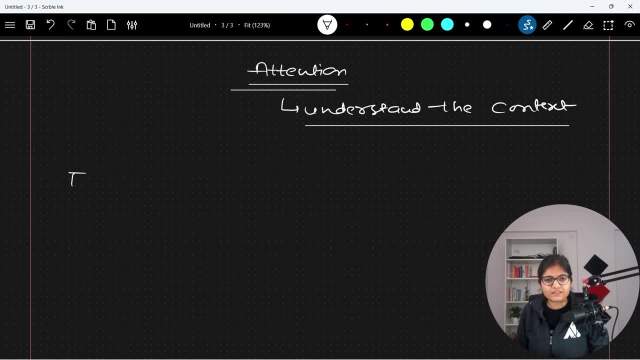 For example. I can just give you one example. I will say the. I will just write one sentence: the chicken didn't cross the road. the chicken didn't cross the road because now, suppose this is the sentence, because it I want the sentence to complete. Now, I told you right, this is the completion of the story, which 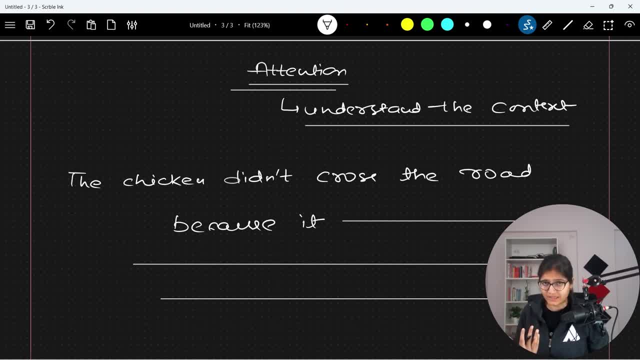 is again an application of transformer which can be easily done by GPT-2, GPT-3 models. Now the question is- but here we need to understand That- how my model will get to know that this. it will represent the chicken or it will represent the road. 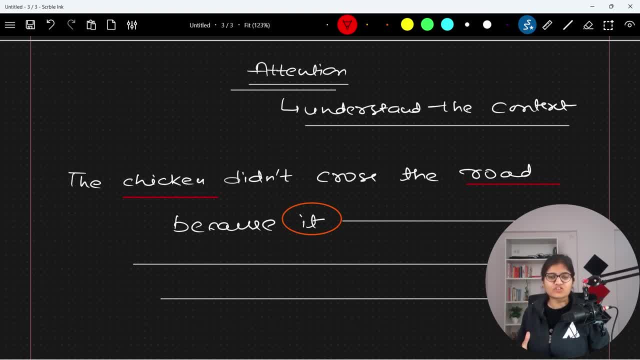 How? So for understanding the contextual part that, okay, this particular word represents the road, or maybe the chicken, then only my model will be able to generate a complete the story out of it, right? And that's where the concept of self-attention or the attention model came into picture. 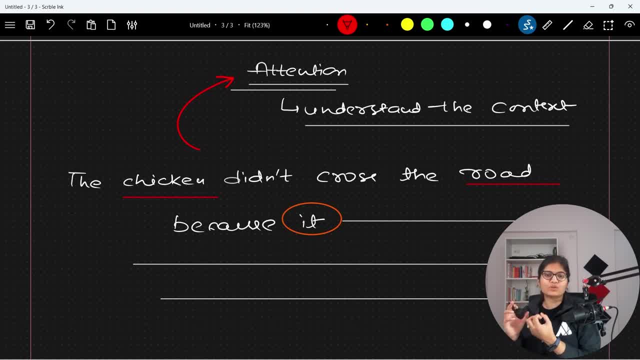 and that is what it is trying to have in their encoder, decoder architecture. specifically in decoder architecture, i would say: attention is there so that it will be able to understand the context out of it, out of the given sentence, and then only it will be able to generate the output. and that's where the biggest you. 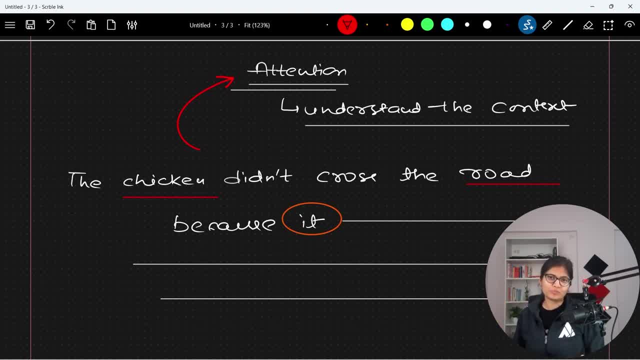 know advantage or the results success will came into picture before that. we do have the different, different kind of techniques to do the same task, but the major problem that we were facing is the contextual understanding in nlp specifically, but afterwards that problem gets resolved right. so that is something that we are, we want, i want to talk about in. 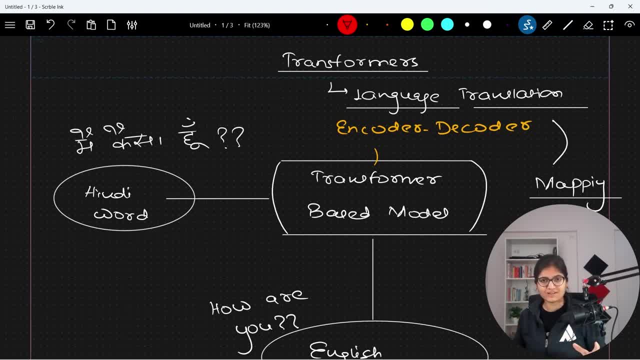 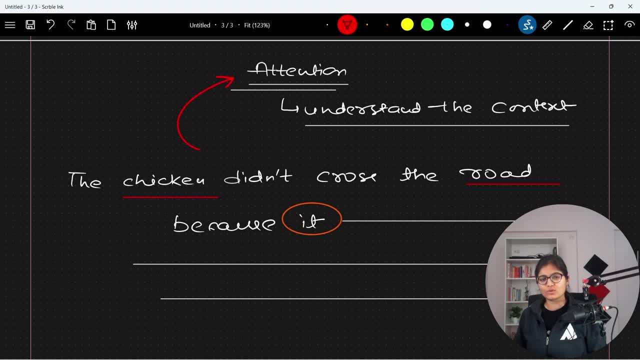 this particular specific session where i just want to give you a transformers architecture overview. now, uh, specifically, you can ask me one question that, okay, you told me that it will be automatically able to complete the sentence, but how is that possible? or it will be possible, or it will be. 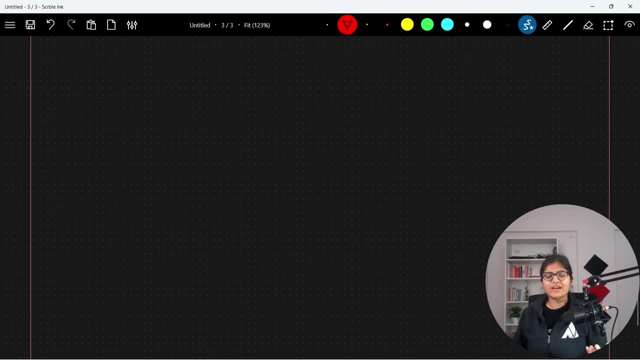 able to do the mapping. how is that possible? obviously, when we are, we are passing it to a transformer model. our model doesn't understand any of the character, doesn't know. i love reading novel. if i'm writing, what is the meaning of i love reading novel? what it will do internally is the very 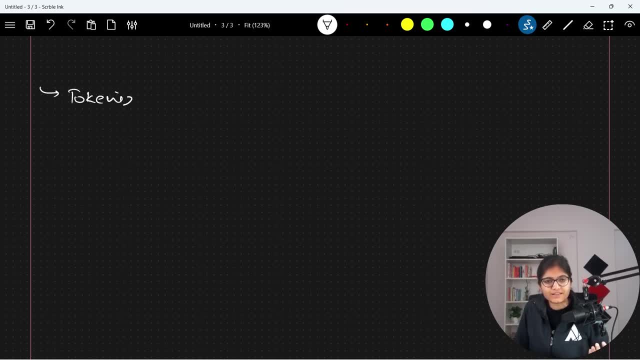 first task is it will try to tokenize the sentences into the words. tokenization of the words will happen and then for every word there is a mapping with the numeric ids, so you will be able to generate a numeric ids out of that. now, after getting this numeric ids, my model: 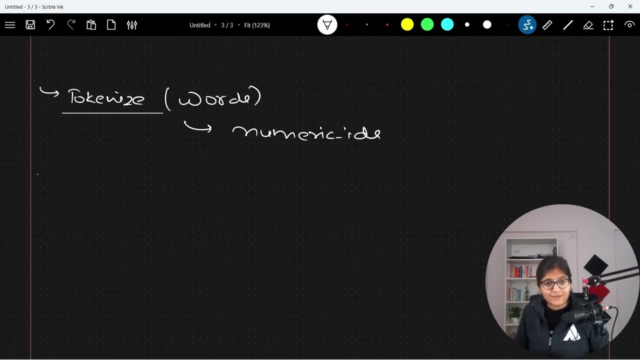 will be easily able to understand the numeric numbers. then we will pass those numeric ids to the model and then my model will be able to understand the context out of it. and that's where the concept of word to vector and all those things, whatever with the word embedding techniques that we have came into. 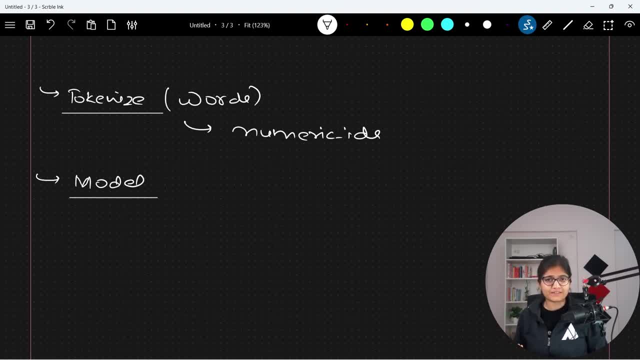 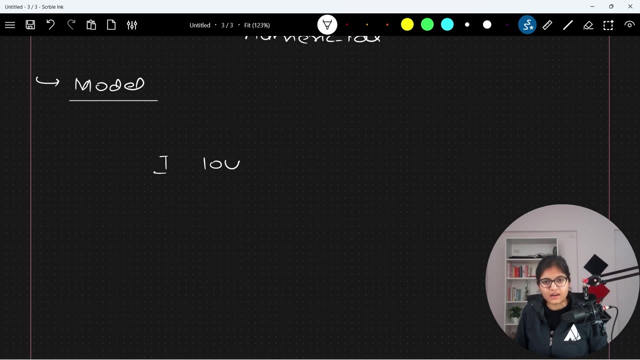 picture, because my model doesn't know what's the meaning of the character that we are using here. what my model know is the numeric numbers and, finally, whichever numeric number is having a higher probability of having a next word. so, for example, if i am saying: i love. 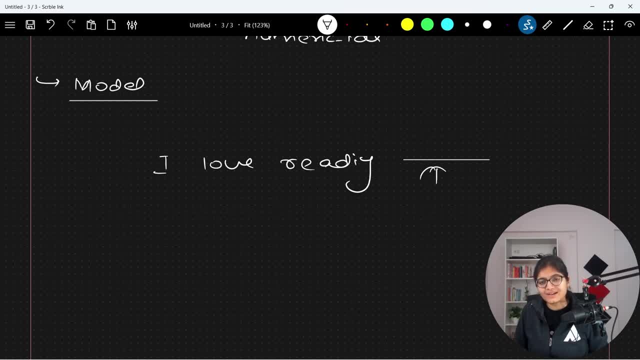 reading now i don't know what is the next word. so what is the next word? is my y? is my y? this is the target value which i want to look for, and this is something which will become the input feature that we have, and this is where the concept of conditional probability came into picture. 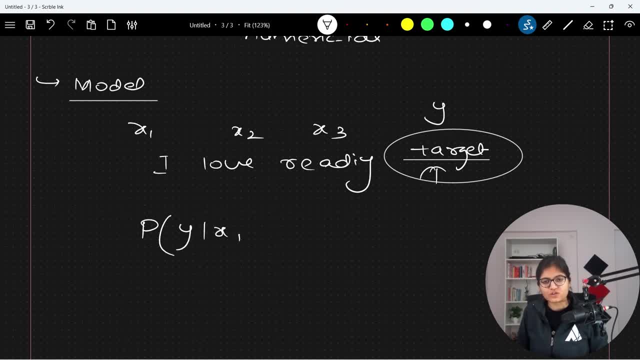 where what we want is: what is the probability of y given x1, x2 and x3 as the input feature? and what we want is: we want that kind of word which is having maximum conditional probability here, which is having maximum likelihood here, and that's where the overall concept 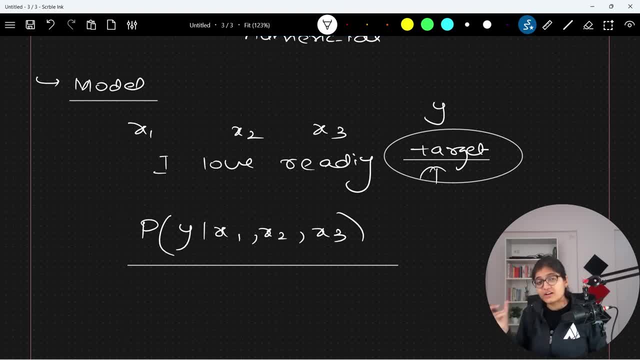 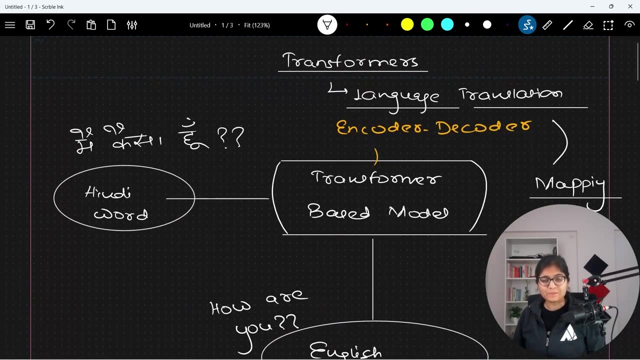 came into picture, and whichever is having a maximum, whichever word is having a maximum probability, that word will become the next, and this is how complete text will be generated in a generative task. right? so this is overall idea behind how the generation will happen. i can demonstrate you one very simple 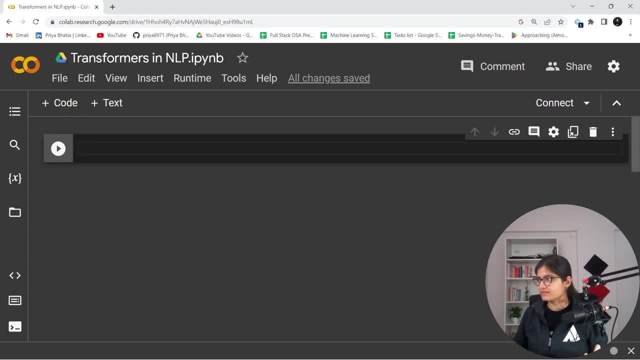 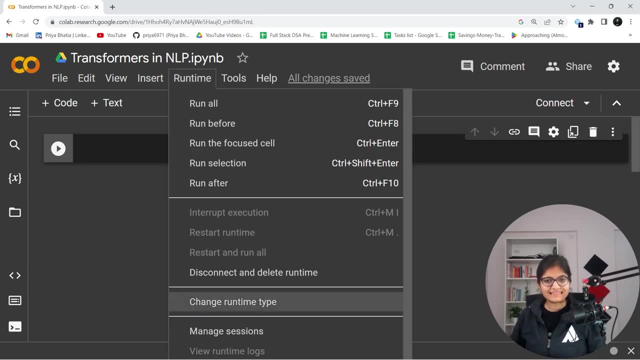 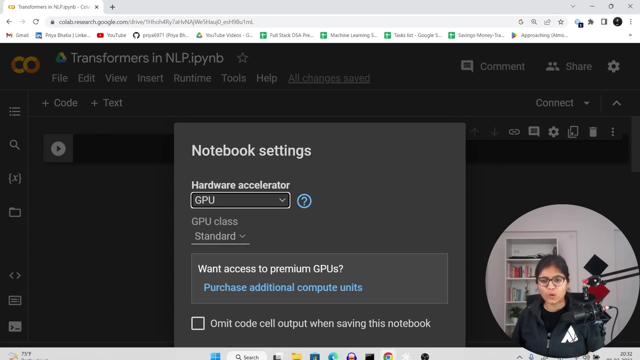 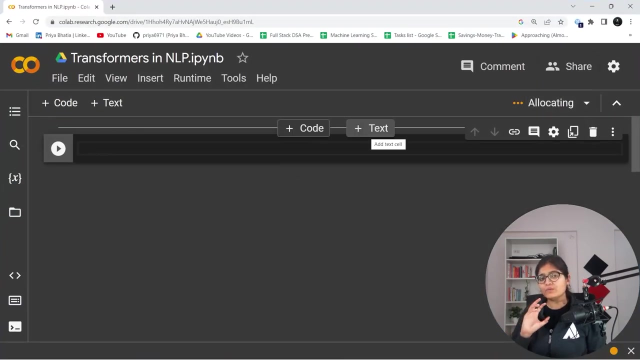 demo here so that you will be able to understand whatsoever uh i am talking about here, but you know, uh, you have to understand the different, different uh, you know hugging face libraries to, oh, uh, to get the overall understanding of the same. just give me one second. i'm just connecting to gpu. what i can do is let me connect it now. 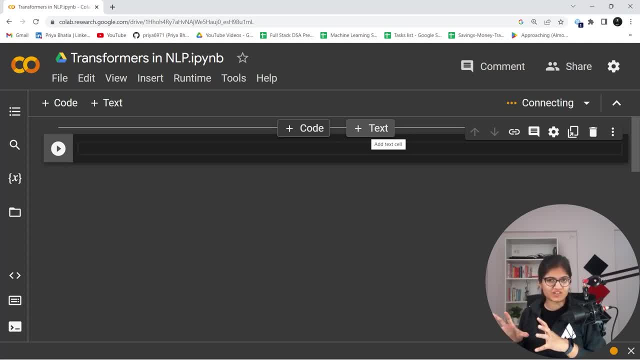 in order to, you know, use any of the transformer based models or any of the pre-trained models in transformers, you need to first of all install the transformers. you need to first of all install the transformers so that you can use any of the pre-trained models present in the 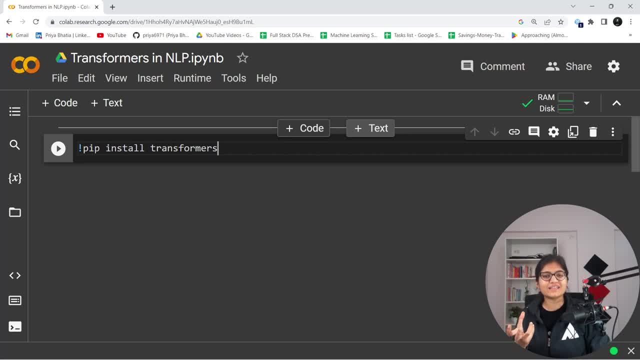 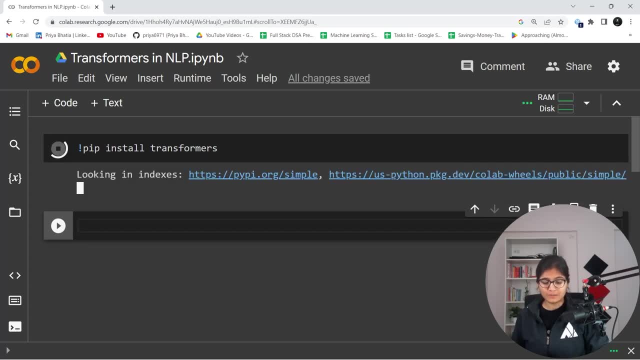 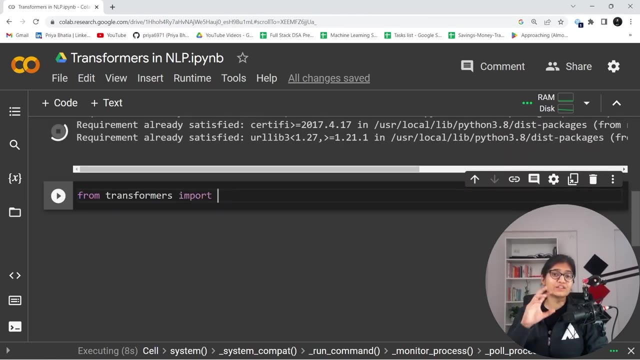 transformers. i would suggest go today and see the list of the pre-trained models that we have in transformers here. if i just install it, it will automatically able to install now from transformers what kind of you know pre-trained models you want to use. you can import that again. there's a huge list. for example, i want to use gpt. 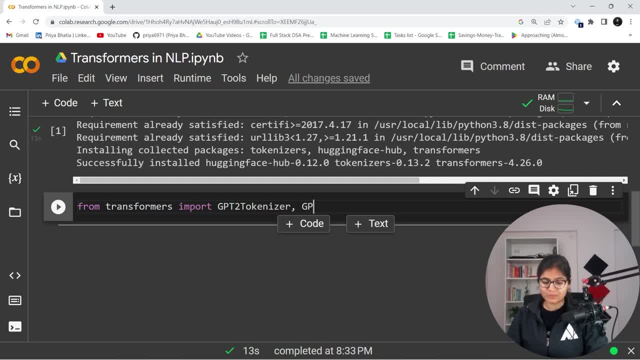 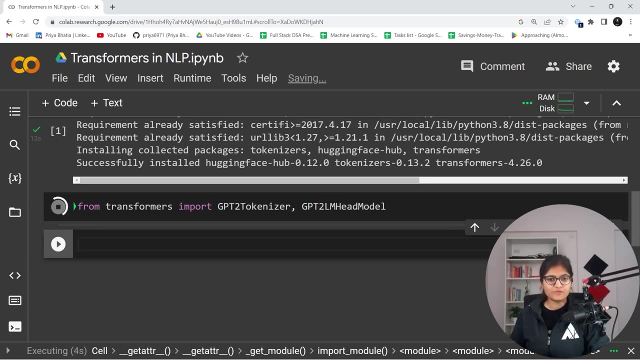 2 tokenizer. to tokenize my sentence, i want to use gpt 2 lm head model, which is a pre-trained model that we have to generate the text so it will be automatically downloaded now. now, after that, what we'll have to do is to create a pre-trained model, and what will happen is: 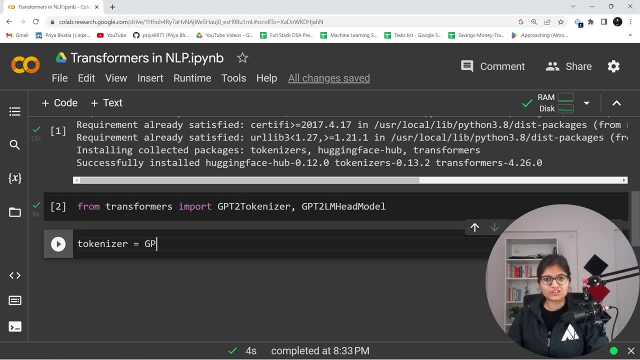 we will be able to directly call the tokenizer here, which is nothing but as equals to gpt, to tokenizer dot gpt2 tokenizer. you need to download that, obviously. so here you need to define: what is that pre-trained model that you want to use? here, for example, i am saying i want to use a 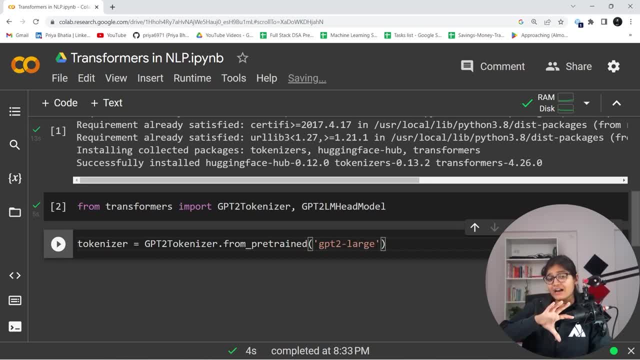 gpt2 large pre-trained model. so if you want to use gpt2 large pre-trained model, this particular model is having a huge number of parameters which has already been trained on and a huge number of huge size of data set which has already been trained on. now, here, if you will observe, 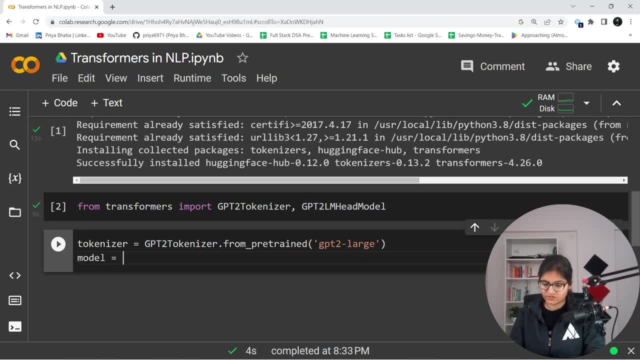 i'll use my model. my model is generative, model is gpt2 lm head model and inside this model, what i will do is, again, i'll call this pre-trained model, which is nothing but gpt to large, and i'll mention the pad token id. 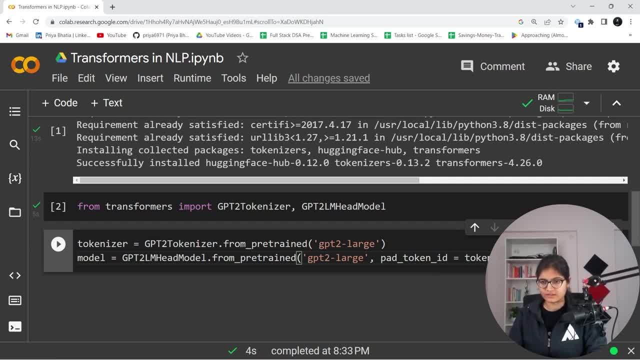 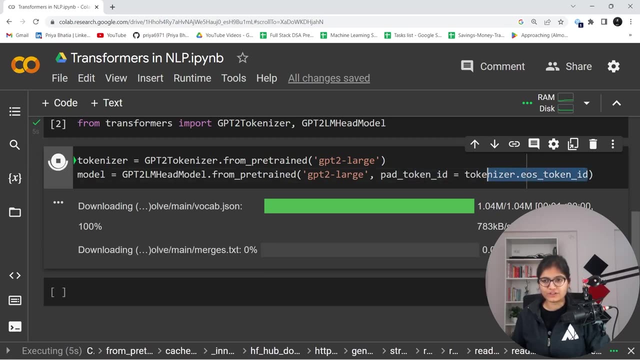 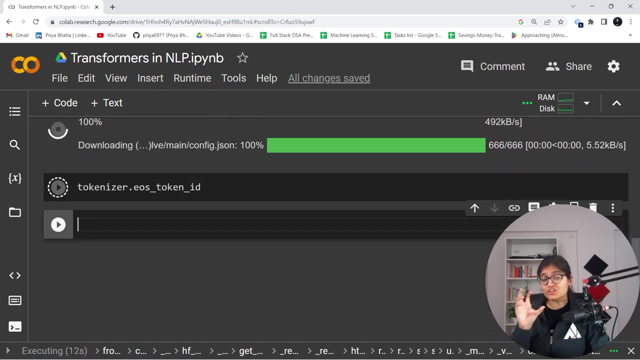 which is nothing but is equals to tokenizer dot. end of sentence. token id. why i'm writing this? because it represents the vocab size. so usually, if i'll just show you the encoding part of this, this much huge is the vocabulary size that we have and for every particular word we will be having a numeric id. 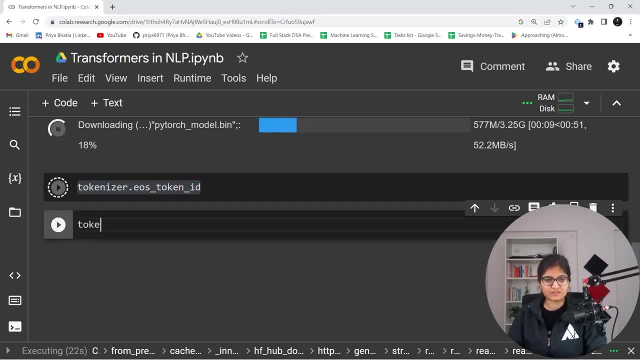 so if i'll just try to decode this, i'll show you this is the indication of the end of text that we have. so let it run. it will take some time and after that i i'll show you that how we can tokenize the sentences. so let me write one sentence here. 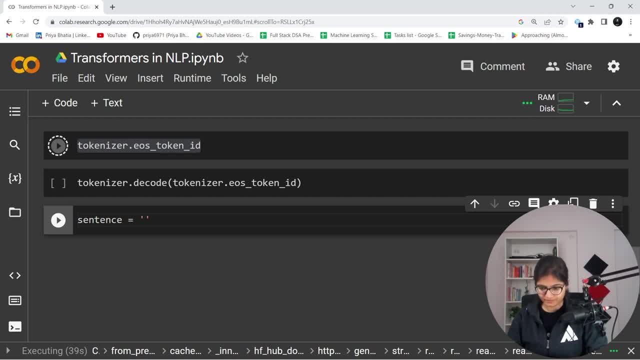 meanwhile, for example, i am saying i love watching motivational movies. okay, this is the sentence that i have, and i want to generate a numeric id out of this particular sentence which i am saying. so what i will do? i'll first of all encode that. the meaning of encode. 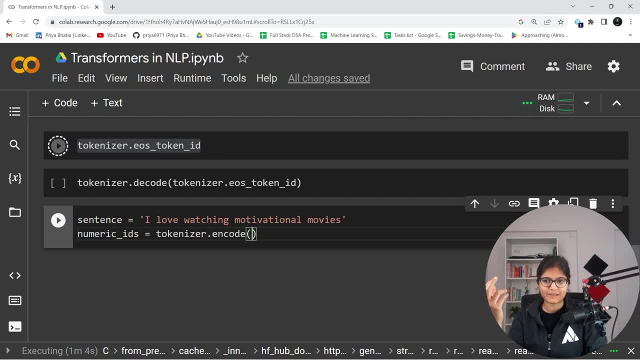 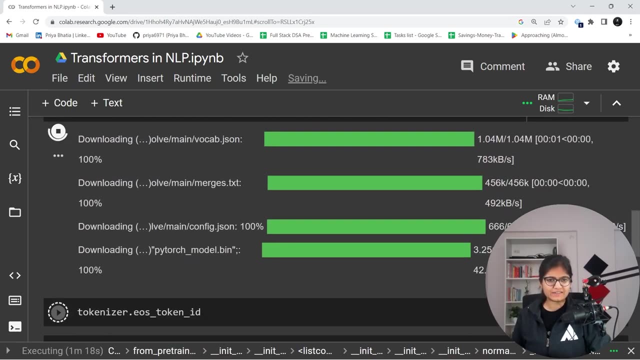 is to convert a character to a numeric id. so what i'll do? i'll pass the sentence and i'll pass what is the return tensor which i want to return it. i want it in the pytorch form, so that is something that we have so see. 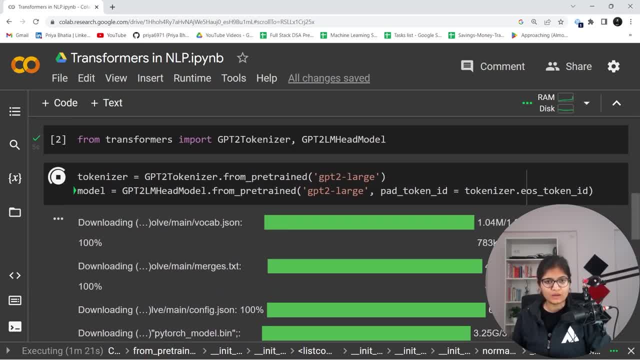 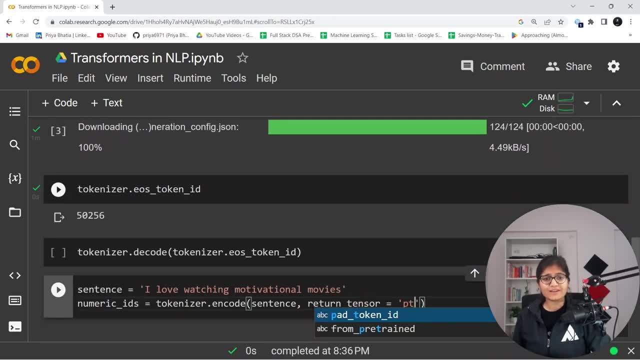 it is taking some time if you have a subscription of collab pro, so it will do much faster job as comparable to what it is doing right now. so here you can see that we will be having a 50 000 approximate vocab size. if i'll just decode it, you will be easily able to. 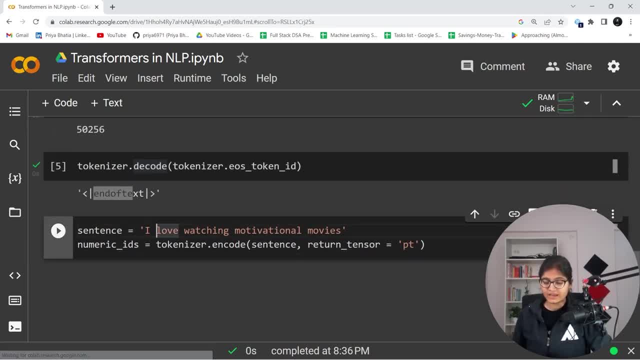 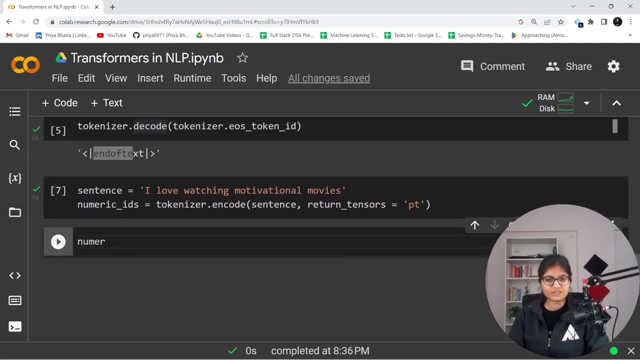 understand that it is representing something called as end of text here. if i just want to show you that, how every particular word is being converted into a numeric id, that's the real object which i want to show you here. so if i just print, what is the numeric? 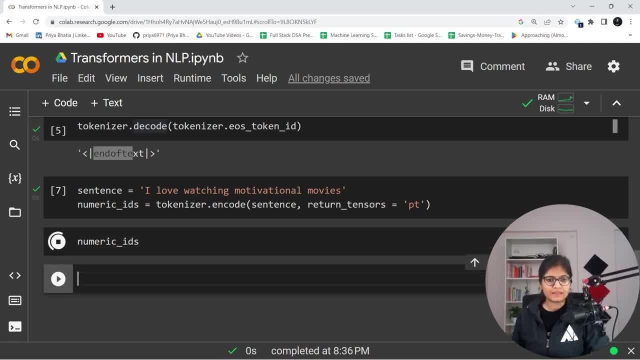 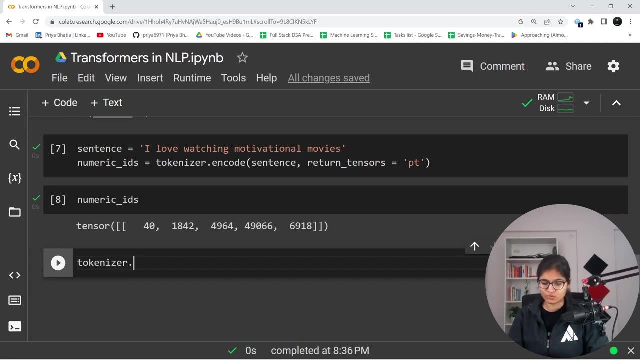 ids i am getting here, then you can see that we will be having 40, 1842, 49, so for every particular character i will be having a numeric id. how can i say that? what i will do is i will say tokenizer, just to show you, demonstrate, you dot decode. and here i am saying: 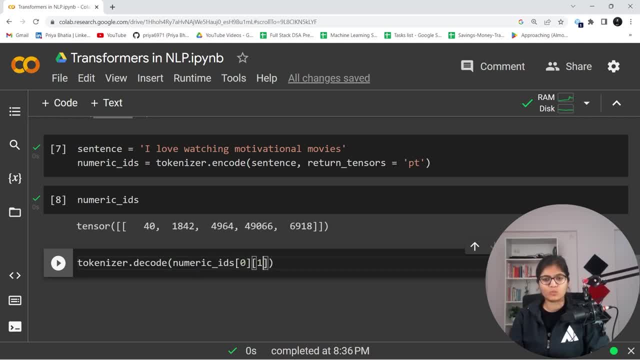 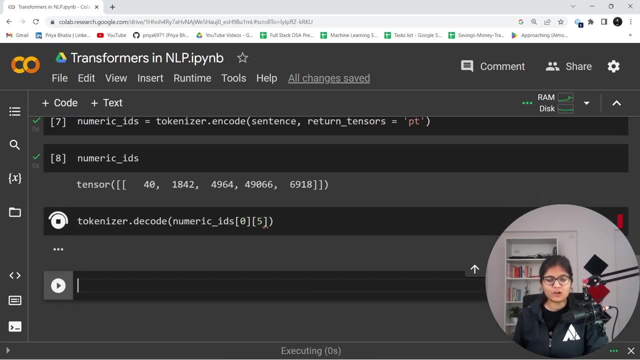 numeric ids: 0, 1, what it is indicating. i think it is indicating, indicating love, right, 1842. if i'll say what is indicating by indication by zero, one, two, three, four, five movies, right? so you will observe that, uh, zero, one, two, three, four, okay, it is four. 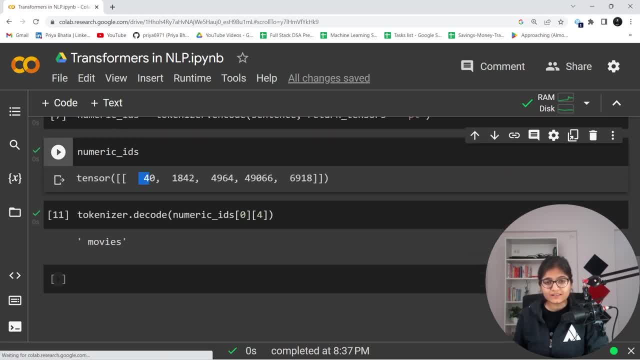 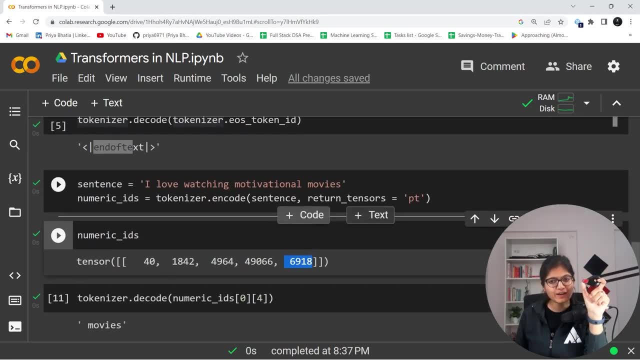 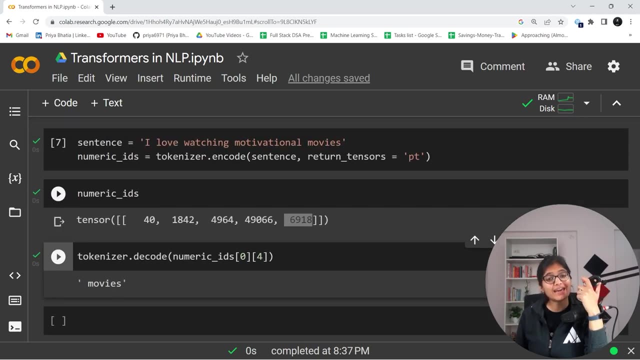 so it will be movies. so you can observe that, starting from zero, one, two, three, four, so we will be having in total five words, and for every five words we will be having corresponding numeric id, and that is what i was talking about for every particular word. first of all is the conversion to a. 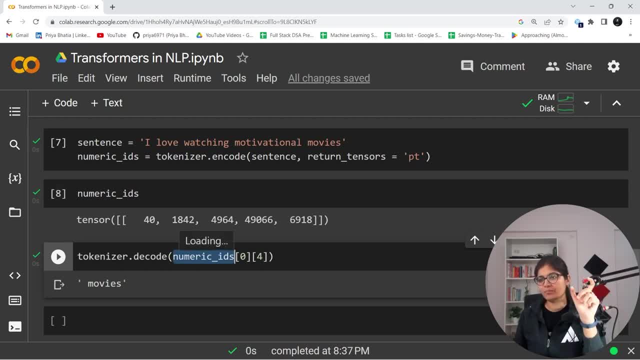 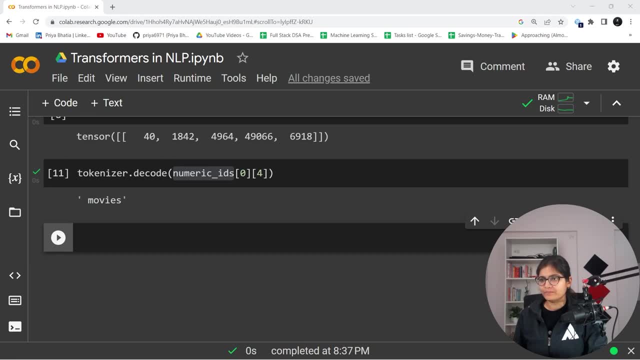 numeric id and this numeric id we will use to pass to the model to generate the further text. now how it will do, let me just show you how it will do. okay, so here you can. you can see that what i am saying. i am passing this numeric. 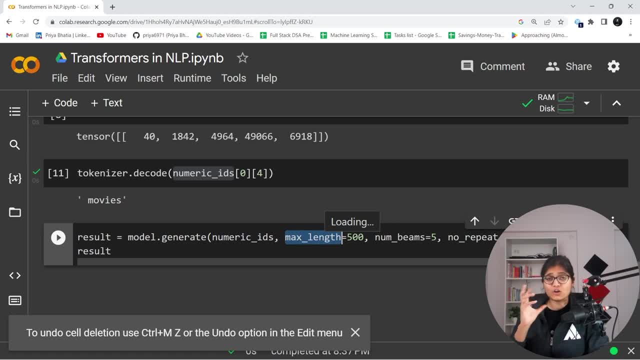 ids here and i am passing what is the maximum length of the sentence which i want. number of beams is just for the optimization purpose as of now, just i'm not going in very much step towards that. just i want to demonstrate you that how the model generation work and how we will be able to 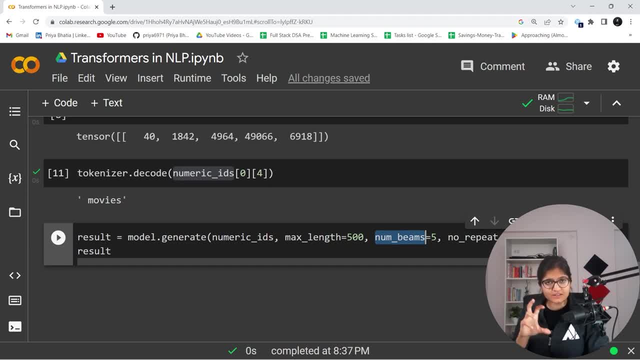 get an output using the transformers, because i have illustrated the concept, uh, theoretically so here, if you will see, if i'll just show you the result here and then, if i decode that tokenizer dot decode, what is the result? i am getting skipping the special tokens equals to true. 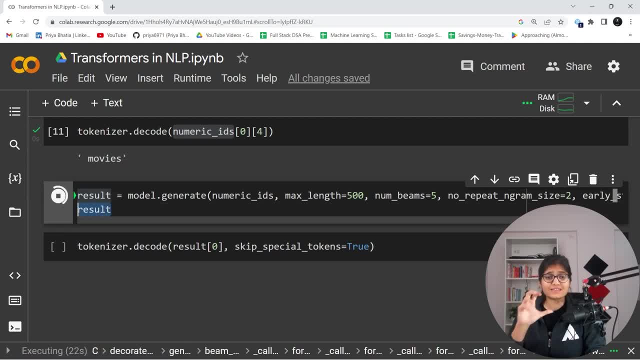 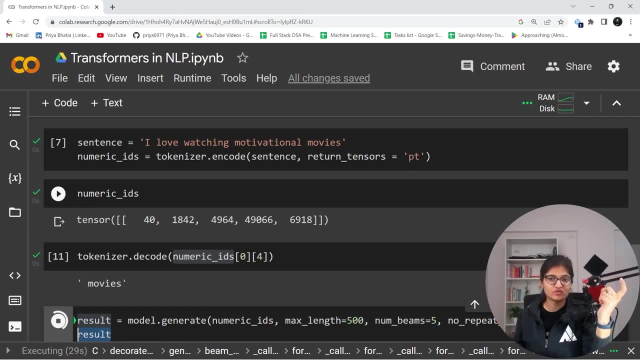 just show you how the result is going to look like. you will very soon see that we will be able to get a complete sentence out of it, and how it is possible only with the help of the transformers. that's the amazing application that we really have in the transformers. that's the capability 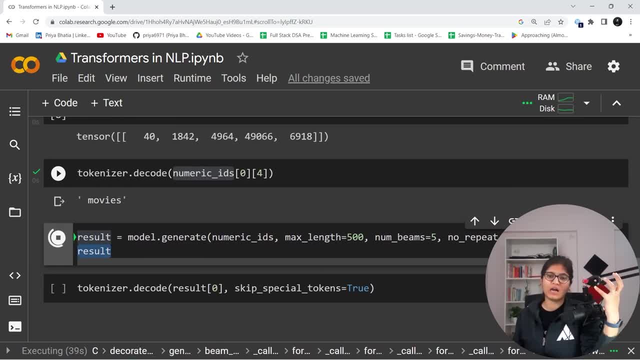 that we have and that's why it is widely used nowadays here. by the way, in the meanwhile, let me talk about the parameters which i am using here: numeric ids. i have shown you that whatever sentence we are picking up, maximum length of the sentence is the maximum length of the sentence, and 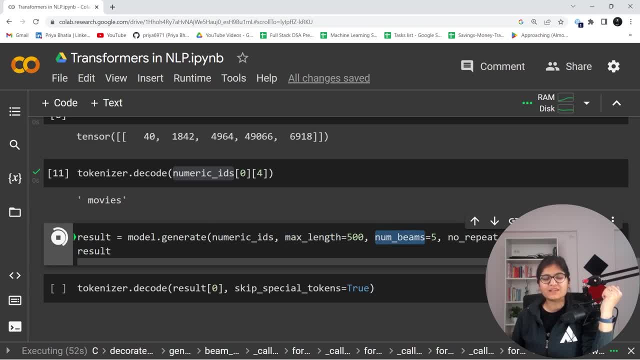 how much is the bigger sentence that you want? number of beams is. it will keep on checking the probability that, whichever would be the next word having the higher probability that would. it will pick up when i am saying five at a time. it will pick the topmost five probabilities and, finally, 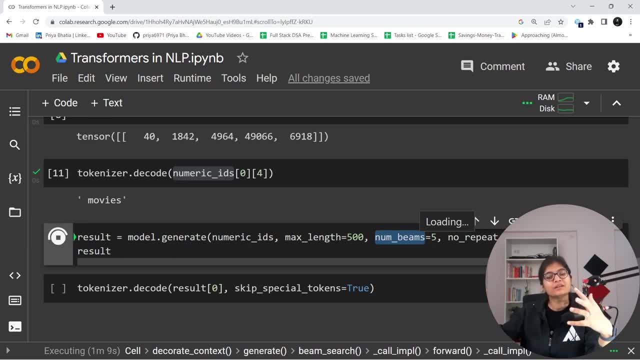 whichever complete sentence sentence is having a higher probability, that particular sentence will be the one which will be the final one. no repeat: n gram size is something which is saying that there will be no. two grams will be matching. there is no duplicacy. early stopping equals to true indicating. 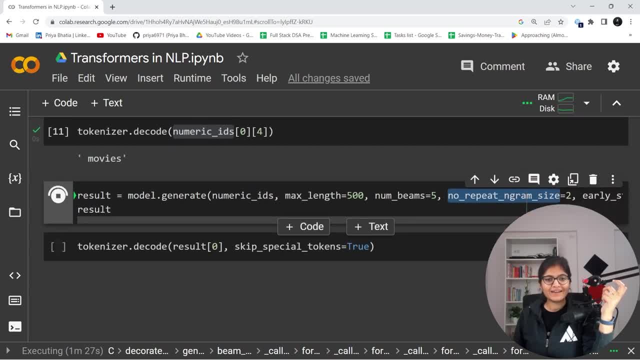 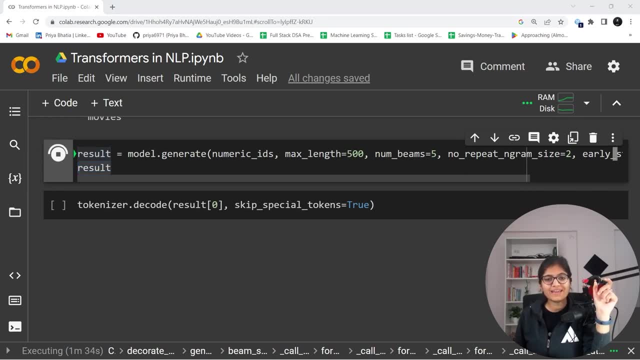 that there should not be overfitting in the model and finally, we will be able to get the result here. you will observe that once you will be able to generate the result, the result will be in the form of a numeric number or numeric ids, but again, for every particular word, we will be able to get the 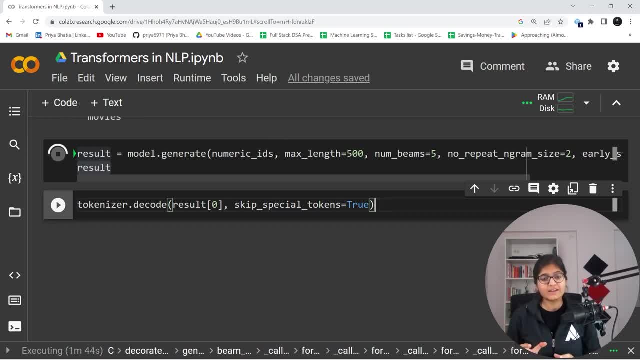 numeric ids, but we don't know the meaning of those numeric ids, right, in order to get what the sentence will be. so what we will do, finally, is we will try to decode it. we will try to decode it so that we will be able to get the final output out of it. so let it run. see, it can take some time. 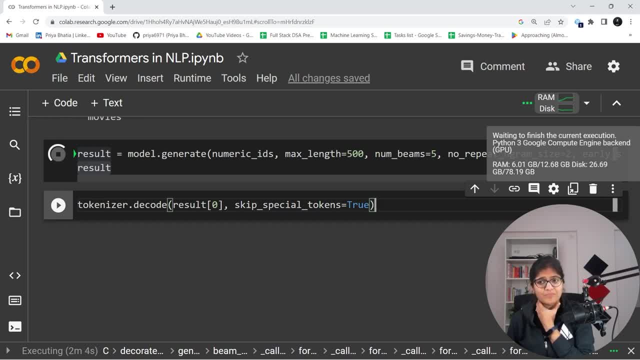 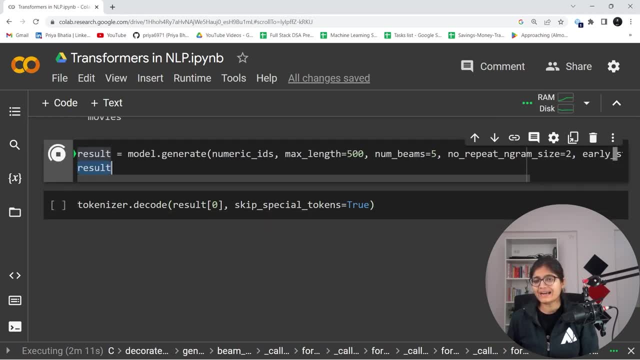 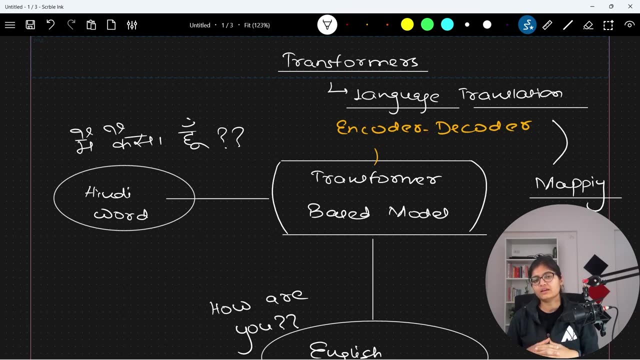 and you can see right, uh, it is using heavily the ram as well and the disk size as well, so let it run. so i hope that you will be meanwhile easily able to get an idea that what a transformers in nlp is all about. so i would say that it's really an amazing, you know uh model, a state of the art model. 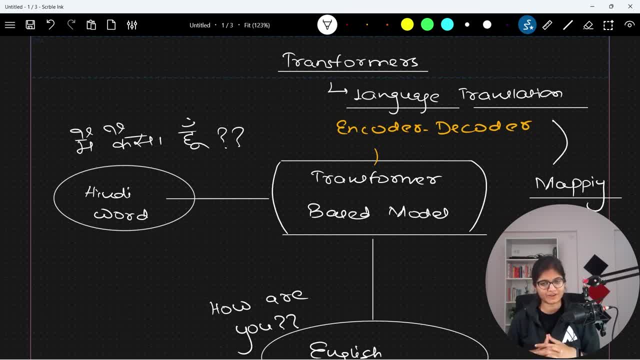 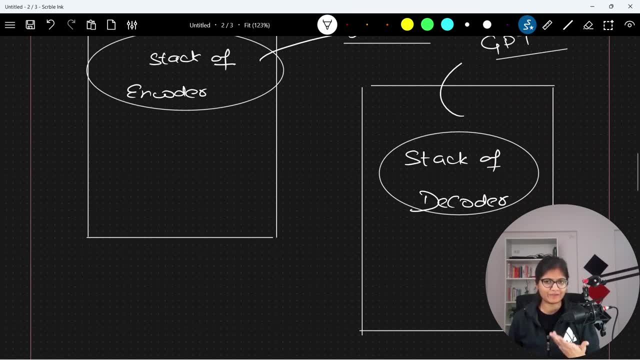 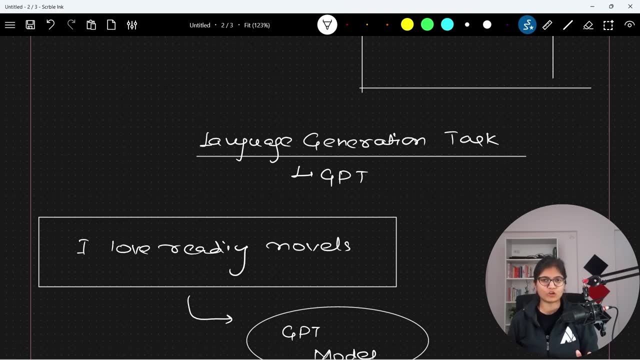 and in the next upcoming videos i will for sure talk about bert in very much depth. i haven't touched upon bert in a depth part, although in gpt i have touched up one and i have shown you the implementation as well, how it will be able to generate the text out of it, basically the foundation. 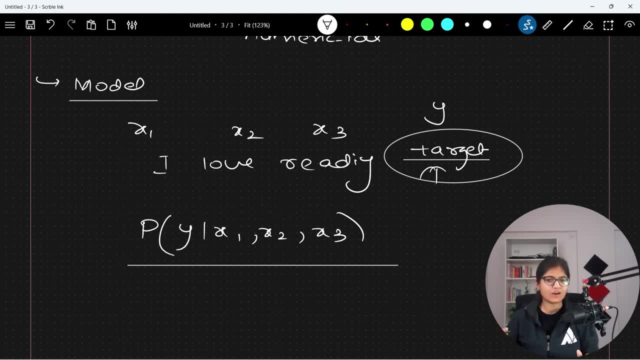 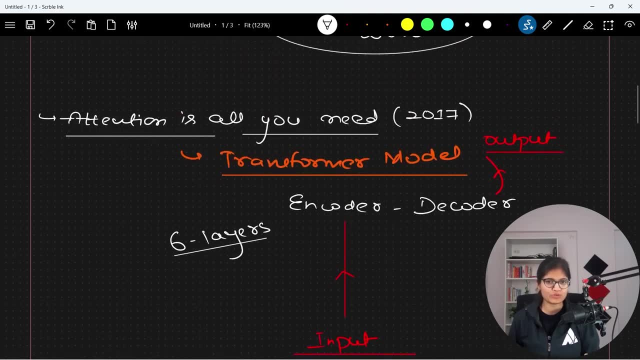 of the nlp. so let's move on to the next step, which is the conditional probability, which i already have talked about, and i hope that you already being aware about what is conditional probability and how, basically, it will be easily able to give us the probability of a target, given the input. 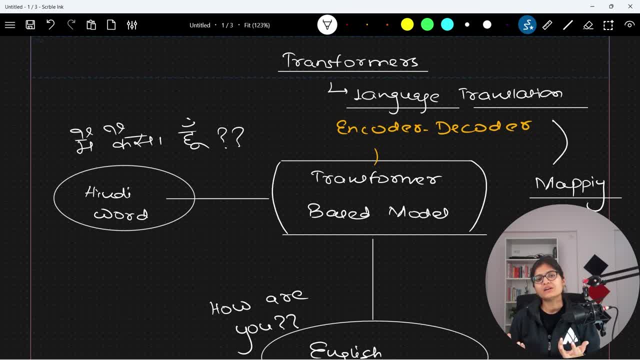 features. you can ask me one more question, that how will i decide how many input features should i take? it should be sequential. you can take three, four, five, according to your own ease, but don't take too much and don't take two lists. depending upon the context size. you can write it down and 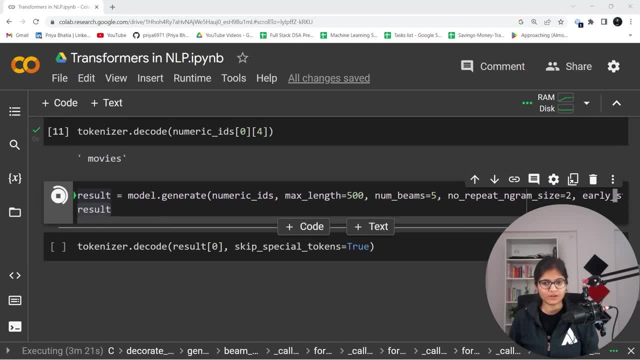 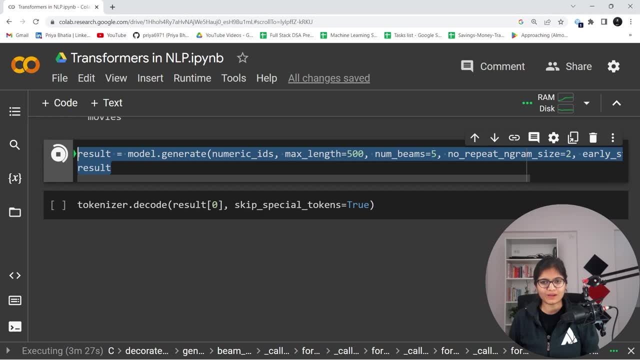 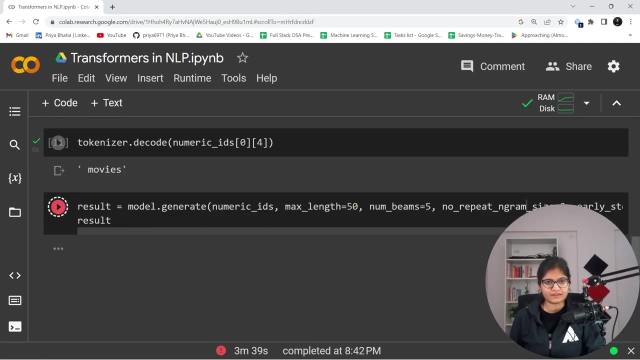 refer. let's see whether it will be able to get or not. so it is taking time. maybe let me do one thing. if i can maybe reduce it to suppose 50, let me just try to stop it and just do it again, if i will be able to get a faster result, i believe. 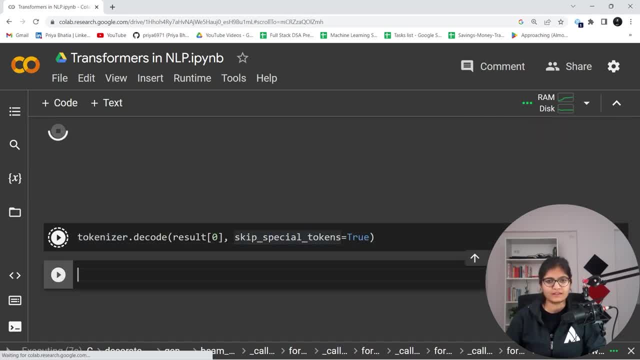 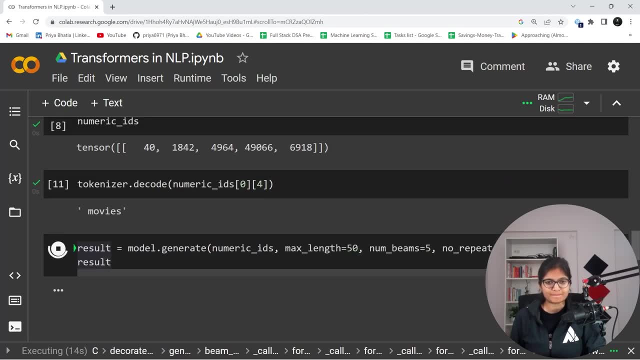 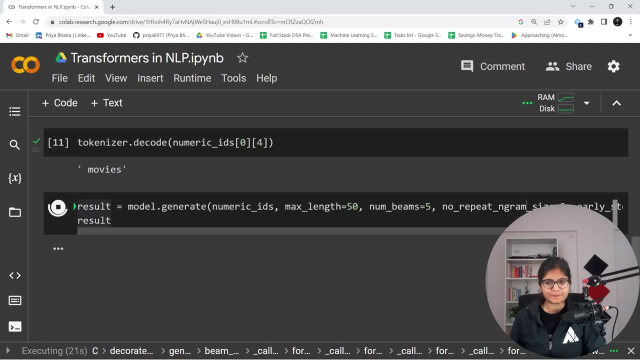 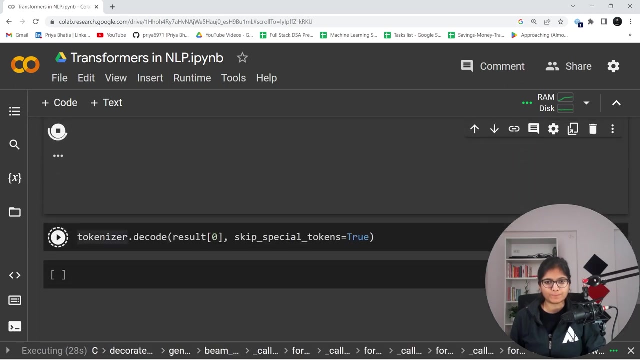 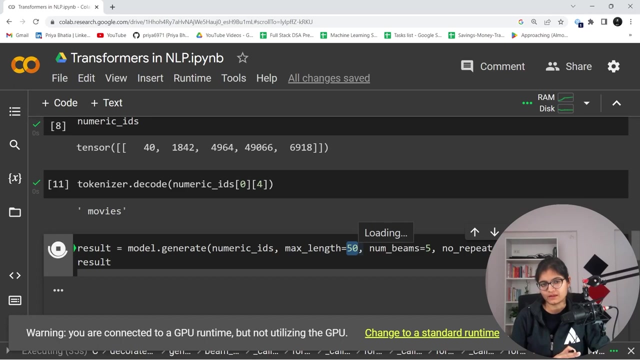 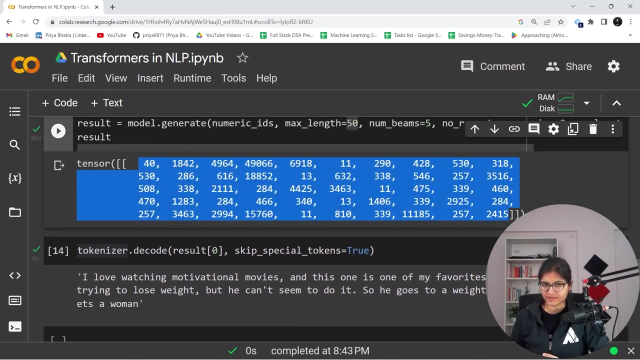 i should, because now the length is only five, so you should take a short, otherwise i have to reduce it to a it to further. you are connect. okay, I am getting the output. I believe so. see, I will be able to get 50 words here, but these 50 words are the numeric IDs again, 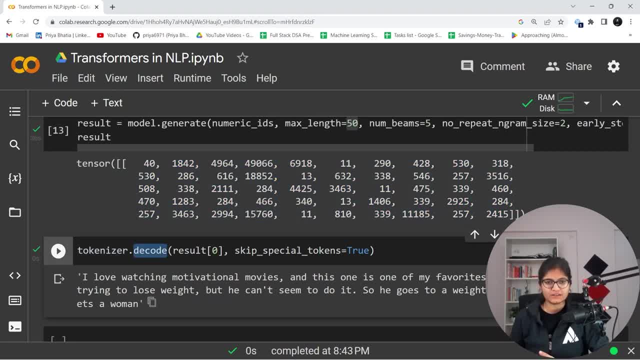 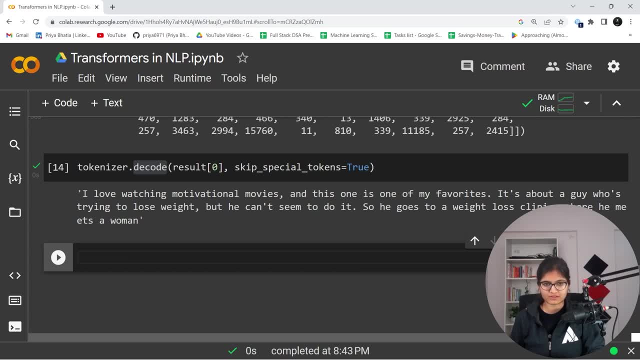 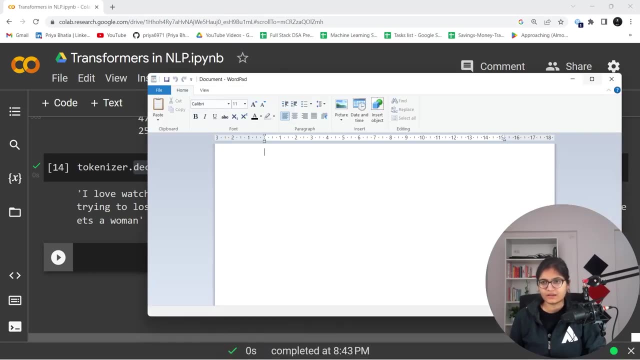 I am getting further. I need to decode that. so if I just copy this and if I just paste it here- not properly visible, so what I can do- maybe I can open a one word pad here and I can show. you see, I love watching motivational movies and 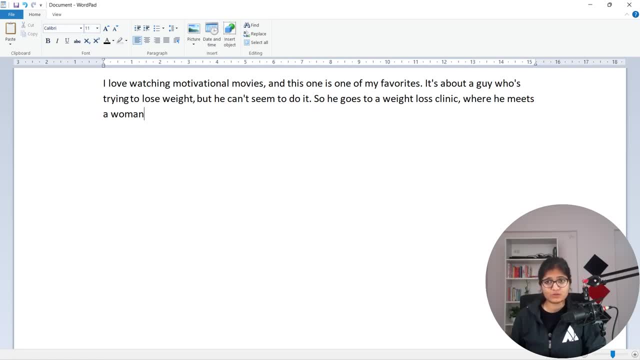 this one is one of my favorite. it's about a guy who is trying to lose weight but he can't seem to do it, so he goes to a weight loss clinic where he meets a woman, and so on. so basically there is a proper story behind it and it seems like. 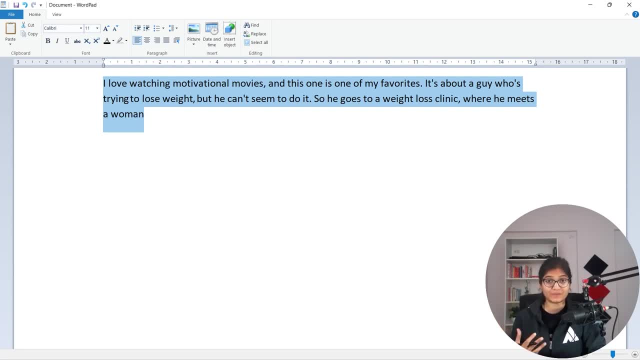 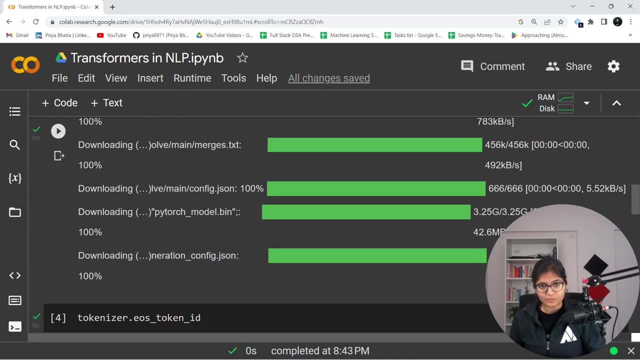 that someone you know human being is coming and telling to me, and that's the power of Transformers, that's the power of training with a huge data set that we have on the web, and this is something which I really want to explain to you all in this particular video, if you still have any sort of doubt regarding 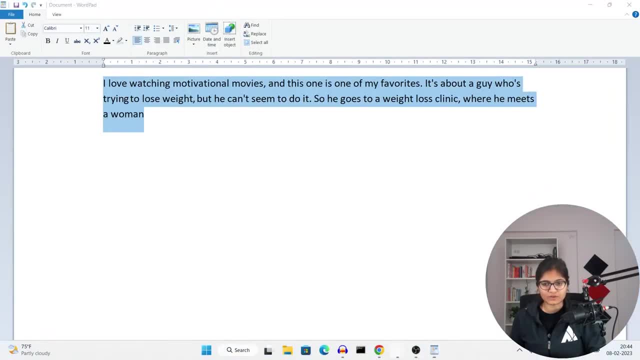 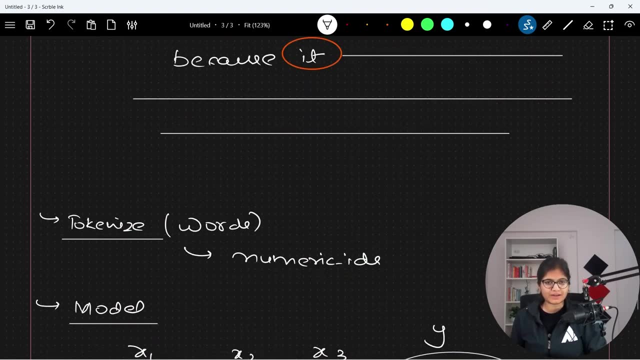 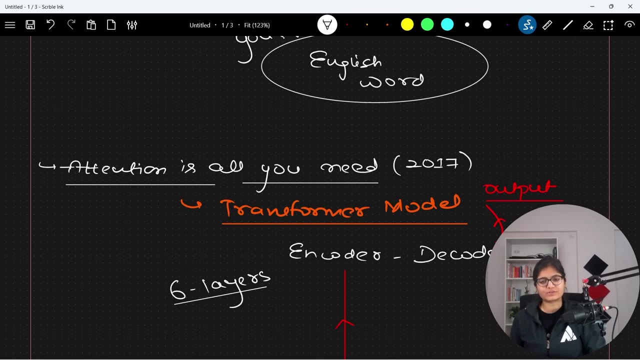 the understanding of how transformers basically work and whatsoever context which I have given you here. please try to go through the research paper. attention is all you need. I have written it down right there. a complete, full fledged architecture is also there. you can go and try to check it out, and there is a